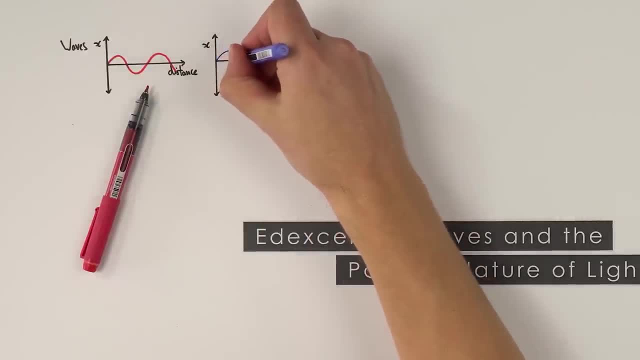 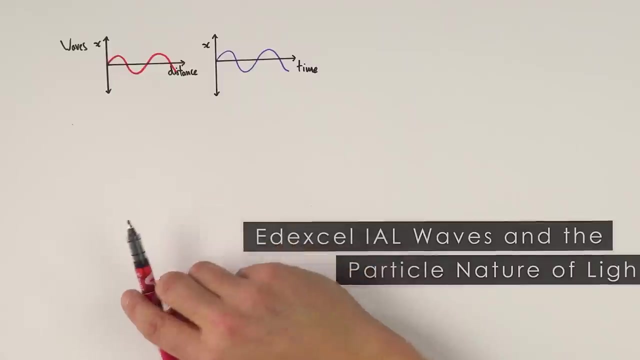 we're going to have time along the bottom, and perhaps this is the behaviour of one particular particle on a wave and how that changes its displacement with regard to time. Now, these are really useful, because what we can do with these is we can actually understand some of the key terms. Now, the first one is the 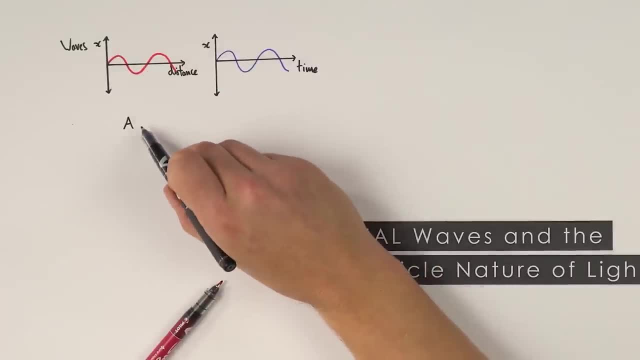 word amplitude. So the amplitude is the magnitude of the maximum displacement from the rest position, and so on. these graphs, it would be this distance over here, And this sequence says the magnitude of the maximum displacement from the rest position, and so on, these graphs, it would be this distance over here. 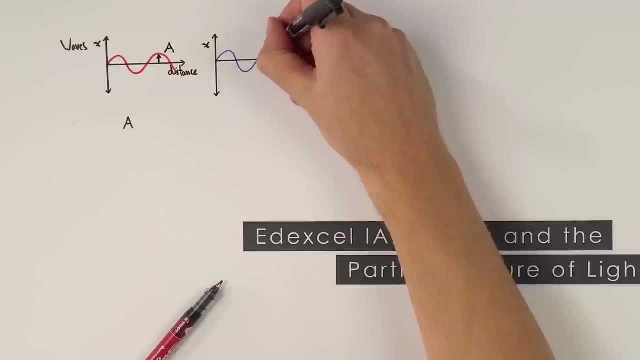 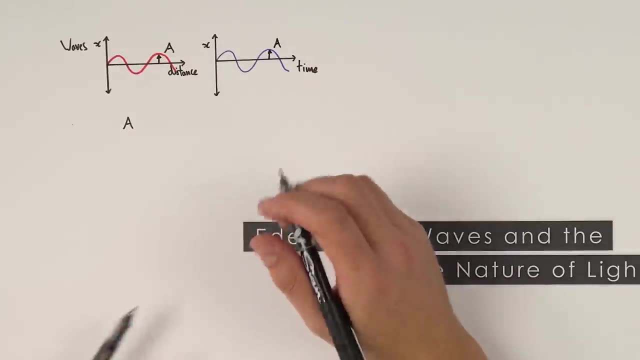 So I'm going to call that a capital A on both of these, And that's how far, perhaps, a particular particle has oscillated away from its rest position. We can also think about the frequency, And the frequency of a wave is the number of complete wave cycles per second. 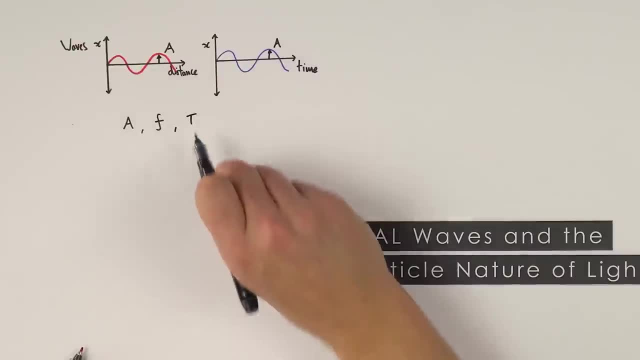 And this is related to the time period, which is capital T. In actual fact, there's an equation that says: the frequency is equal to 1 divided by the time period, And we measure the time- as always, because it's an SI unit- in seconds. 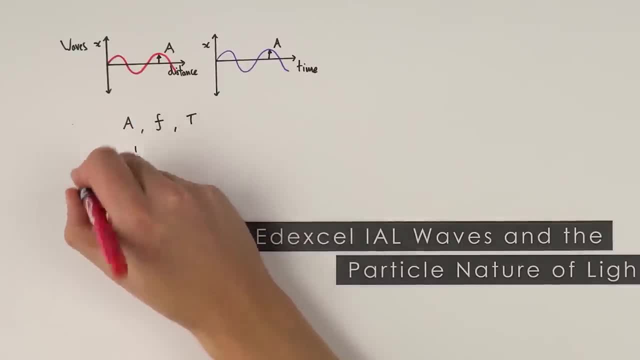 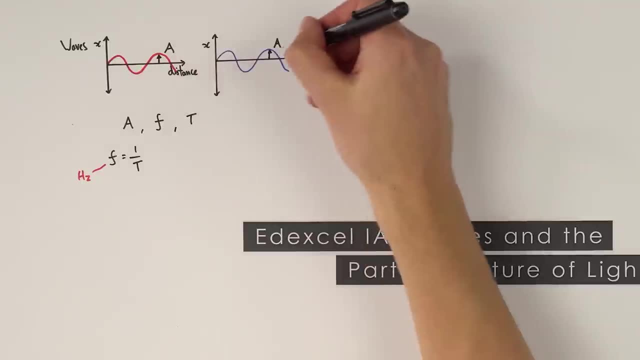 And this then gives us our frequency in the unit of hertz. So the time period is the time for one complete oscillation of a wave, And if we were to look at it on this graph here, if we were to maybe look at one complete wave cycle, 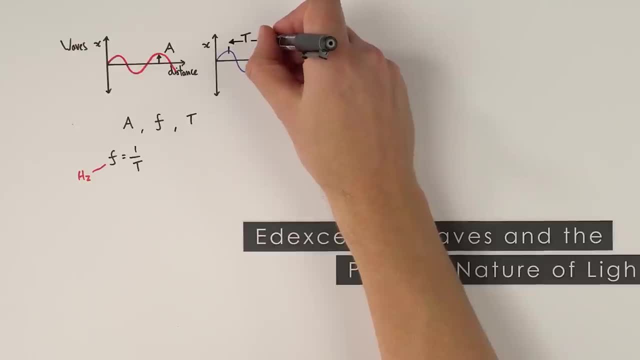 the time period T is a Distance between these two peaks. Potentially, that might be the kind of thing that you might measure on an oscilloscope. We also have the wave speed v, And this is the rate of movement of the wave. 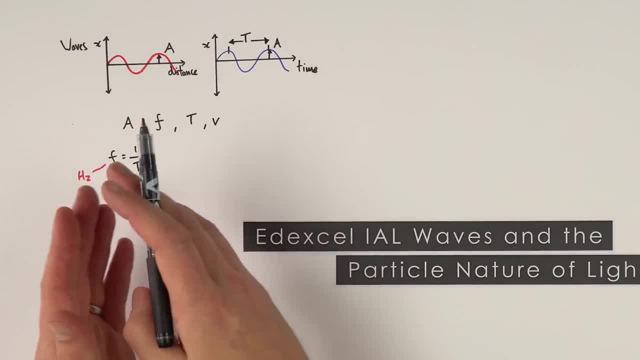 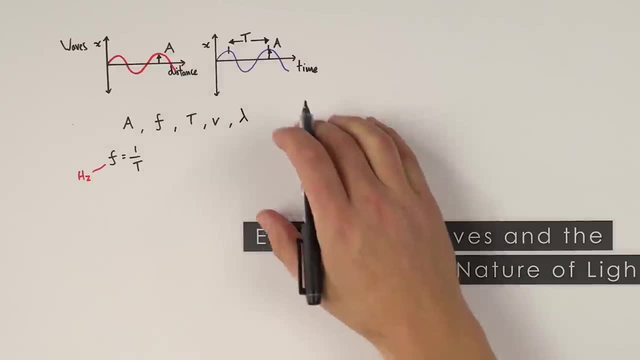 And this is where we talk about waves being perhaps progressive, where they're transferring energy from one place to another. So that's how quickly the wave is moving, And the other term that you'll be familiar with- and often this is from before you started your A-level physics- is the wavelength. 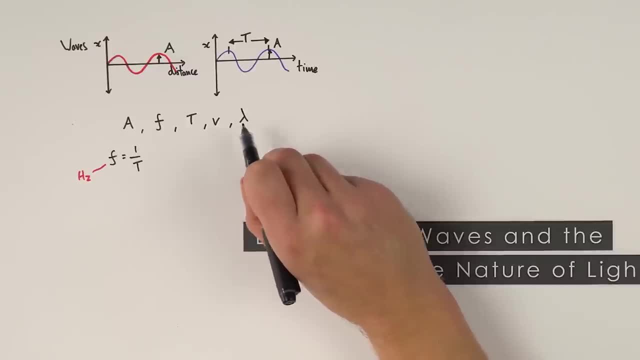 And this wavelength has the Greek letter lambda, And we can think about the wavelength being the distance from a peak to a peak on this graph over here, And indeed, when it comes to measuring the wavelength or the time period, we can go peak to peak, we can go trough to trough. 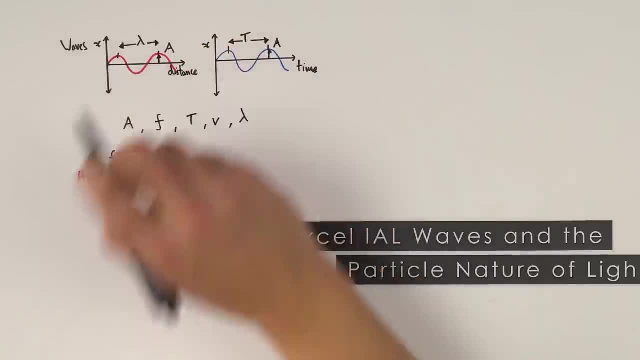 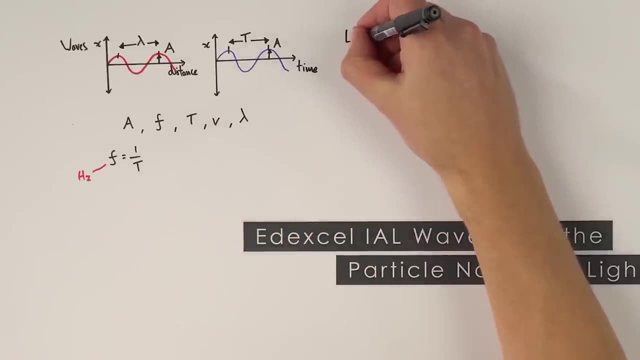 or any point to the next similar point on the next part of that wave. And both of these graphs here can be used to represent both longitudinal and transverse waves. Now both of these sorts of waves can be demonstrated in the following way: Demonstrated in the lab using a slinky that long spring. 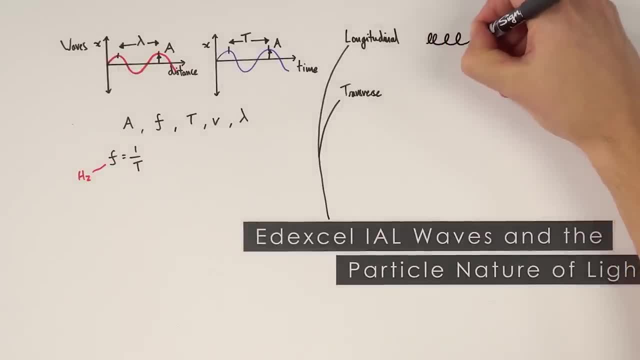 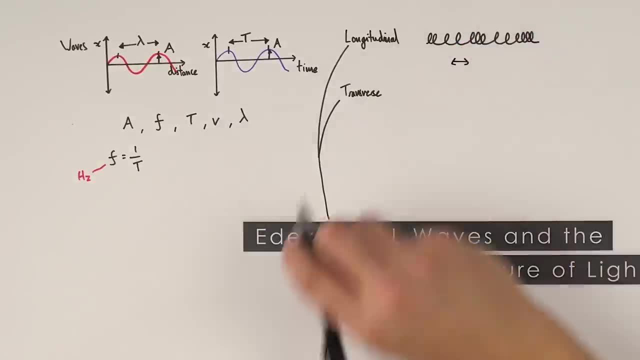 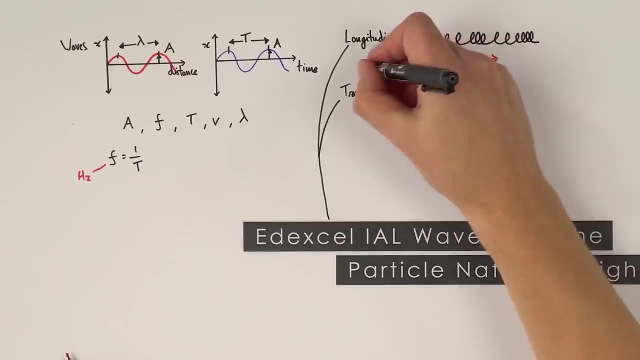 If you have a longitudinal wave, we get something that looks a bit like this, And for the longitudinal wave, the slinky is moving back and forwards, And this is also the same direction as the energy is transferred from here to here. Now, examples of longitudinal waves include things like sound, ultrasound. 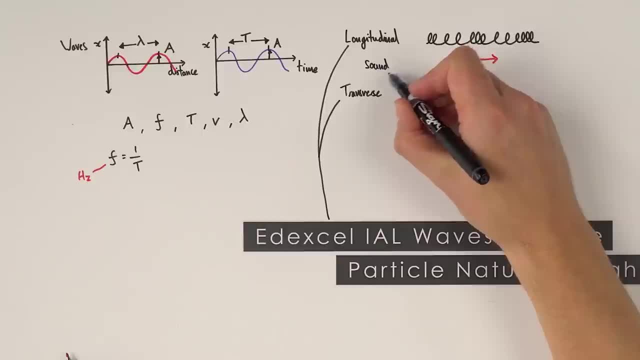 And these are waves which are mechanical because we have particles which are oscillating. In actual fact, if we were to look at a sound wave, what we might see is that the air particles are oscillating backwards and forwards And we have particular points where we have more air particles. 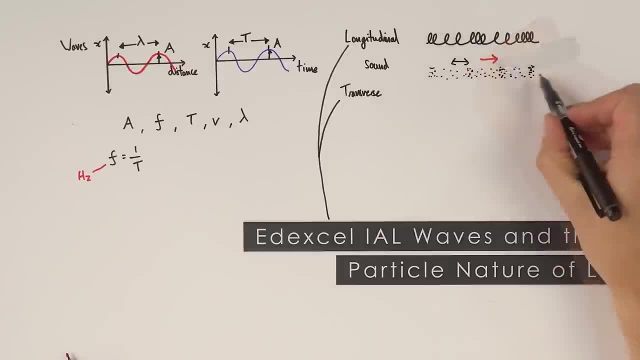 then they become more spaced out, Then we have a region a bit like this, And effectively the distance from this point to this point is going to be equal to the wavelength of that sound wave. So when you have sound, ultrasound, other longitudinal mechanical waves, 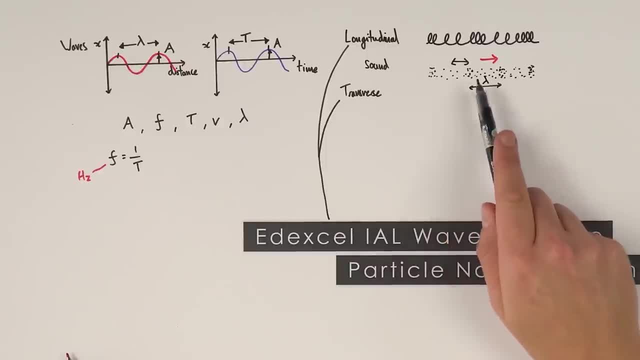 we have areas of compression. So when you have sound ultrasound, other longitudinal mechanical waves, we have areas of compression. So when you have sound ultrasound, other longitudinal mechanical waves, we have areas of compression and rarefaction. And it's not: the particles are moving from one place to the other. 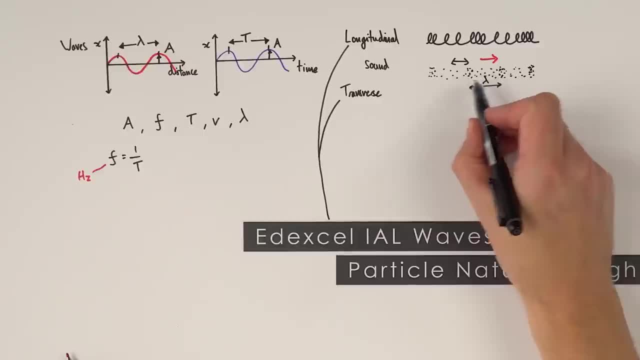 The particles are just oscillating, but parallel to the direction of energy transfer, So that's a longitudinal wave. The other kind of category of wave we have is transverse and often, if we see it on the slinky, this is when you move the slinky side to side. 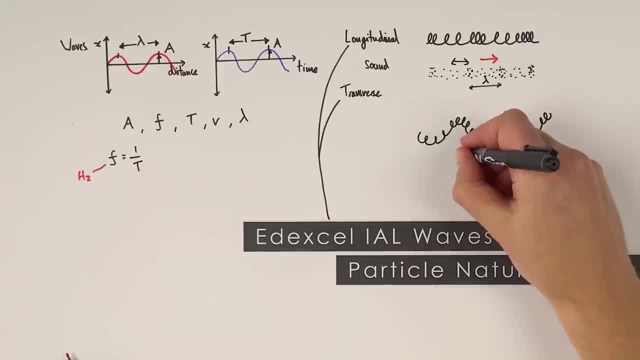 rather than back and forwards, And what we have now are the oscillations. or the wave is moving side to side, or the wave is moving side to side, But here the energy's transferring here. But here, the energy's transferring here. 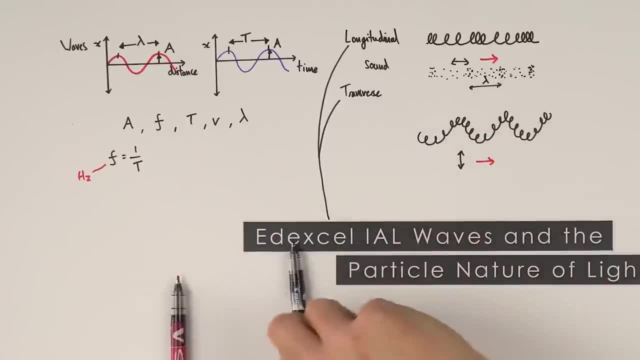 But here the energy's transferring. here the energy is being transferred from here to here. So now, when you have a transverse wave, the oscillations are perpendicular to the energy transfer, And here the oscillations could be particles which are moving up and down. 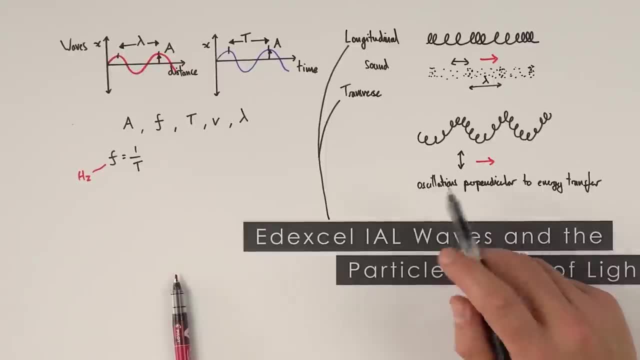 or it could even be the oscillations in electric or magnetic fields, And this is when we come onto our electromagnetic radiation. Now we can do an experiment to actually investigate the speed of sound in air, sound being a longitudinal wave, And this is one of the core practicals. 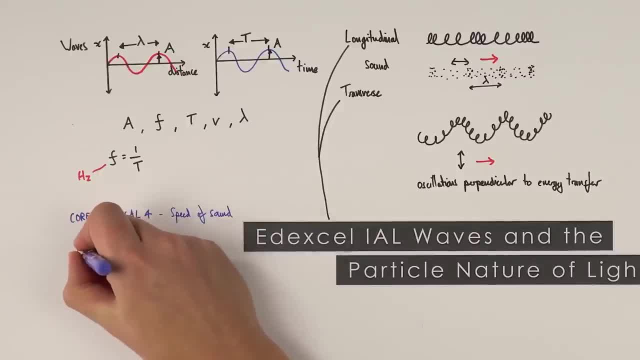 Now, there are various ways you can actually set this up in the lab, but effectively what we have is some kind of loudspeaker, And this is going to be emitting a sound wave. You then have two different microphones, And if you were to measure the distance between them, S. 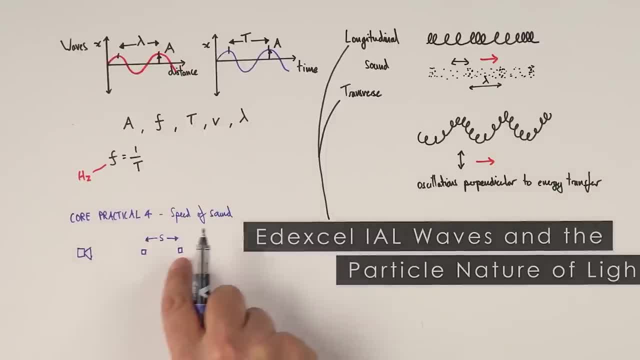 you can then send a sound wave that gets picked up by this microphone and then by this microphone, And the way we actually detect that is using an oscilloscope, And what you can do is you can input into the oscilloscope both of these microphones. 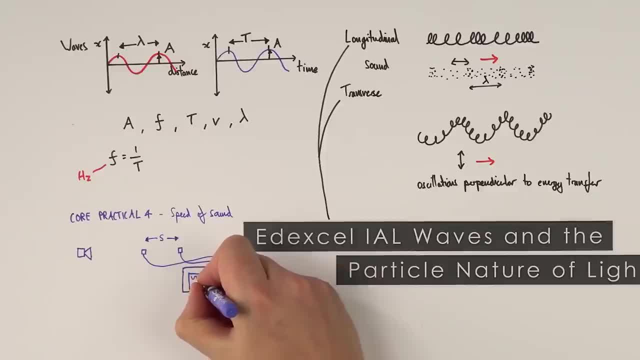 And what you'll then see are two different signals, And by lining up the two signals you can then look at the time difference between the wave hitting this microphone to this microphone, And then you can just use the equation that says speed is equal to the distance over time. 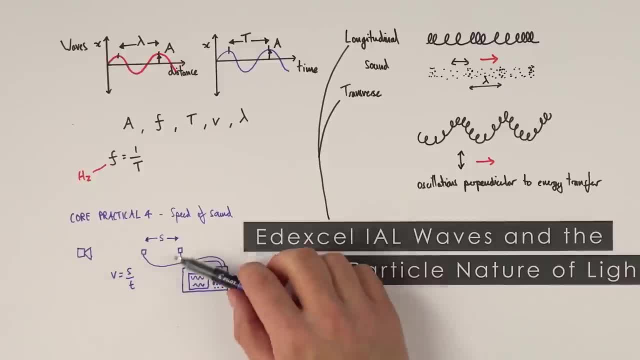 to actually work out how quickly that sound is going, And it's going to be in the order of 300 to 330 meters per second. But again, there are various ways of carrying out this practical. Now, with this topic, there are going to be a lot of new words. 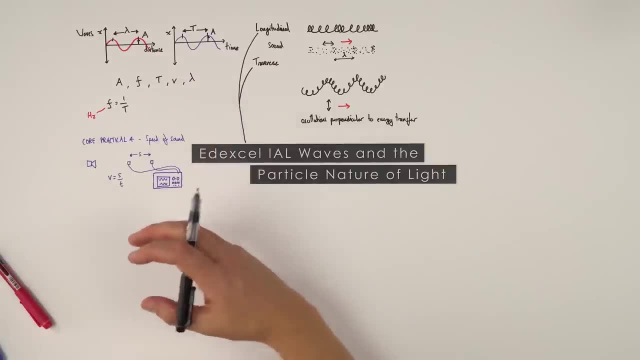 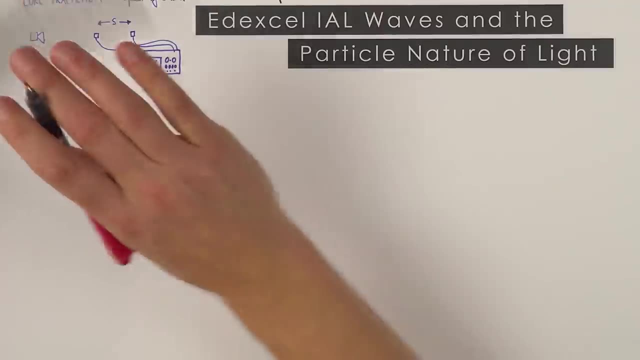 These ones here you will be familiar with, but we have some other words that you need to understand what they mean, And we can actually represent waves in many different ways. So sometimes you might draw a ray of light, perhaps using a ruler, And we can show that that's a straight line. 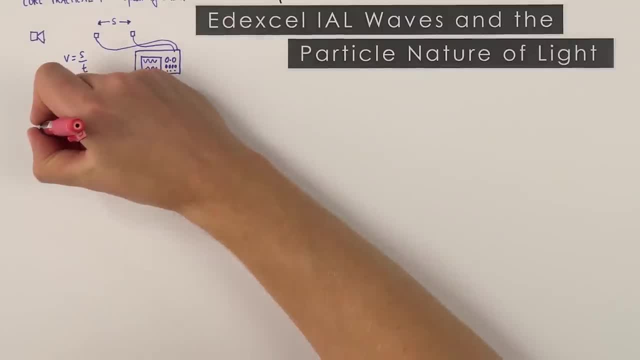 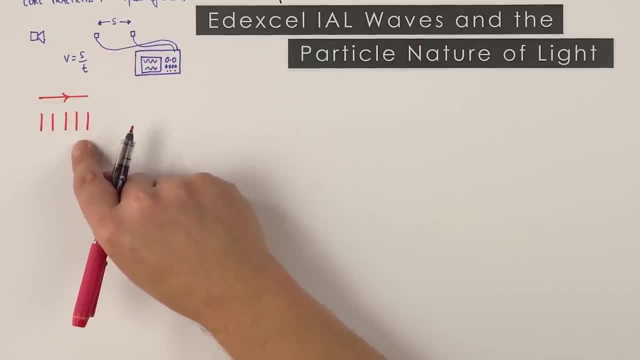 as a wave is moving from one place to another. The other way we can do it is we can actually draw the wave fronts, And this is another way of representing that wave And, as we've seen up here, we sometimes draw the waves like this: 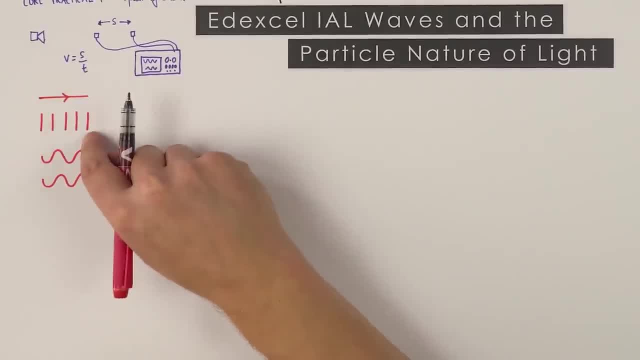 And we can maybe think of the wave fronts as being the top-down view of the water ripples that you might see in a ripple tank, And here that wave front is a position where all of the waves here are in the same phase position, So this might be the peak of one wave. 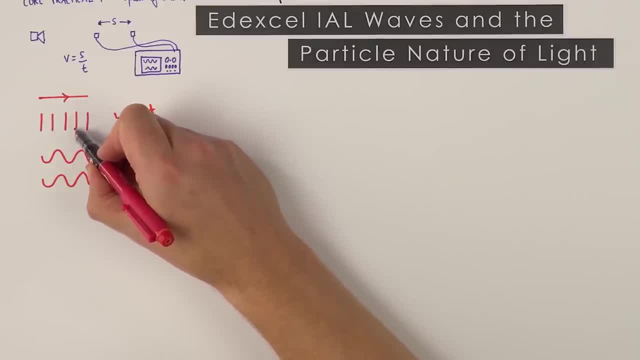 And at this point here all of those parts of the wave are in phase, And again that's going to be the peak of that wave. The other thing we can think about is something called coherence, And here we can maybe talk about two different wave sources. 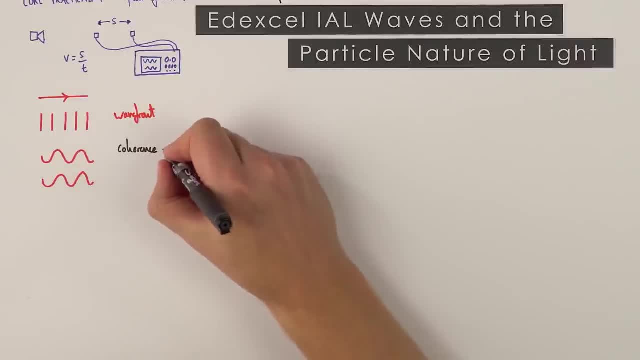 Now the waves are going to be coherent if they have the same frequency and also a constant phase difference. So that means they're going to have the same wavelength and often they have similar amplitudes, And that's really important when you come onto some of the work looking at diffraction later on. 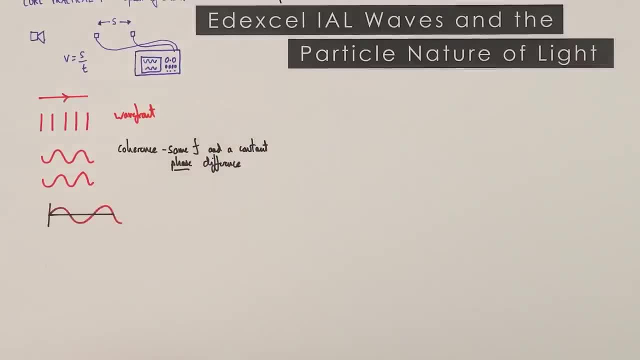 So we've got the same frequency and a constant phase difference. But what do we mean by phase difference? Well, it's to do with which part of the wave cycle that wave is in. Now, if you have one complete wave, that's going to be equal to 360 degrees. 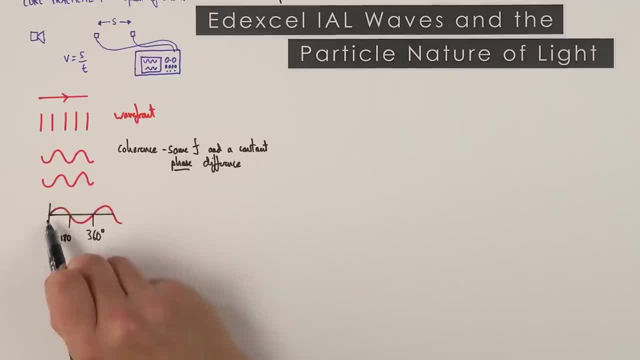 Half a wave cycle is going to be equal to 180. And then a quarter of a wave cycle is 90, and so on. Now, often when it comes to physics, we don't just use degrees, but we also use the radian. 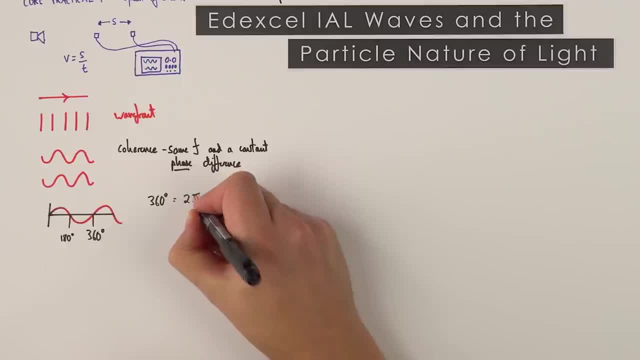 And you might recall that 360 degrees is equal to two pi radians. Now, the other thing we can look at when it comes to waves is the difference between two different waves and how far they've travelled, And that's where we have path difference. 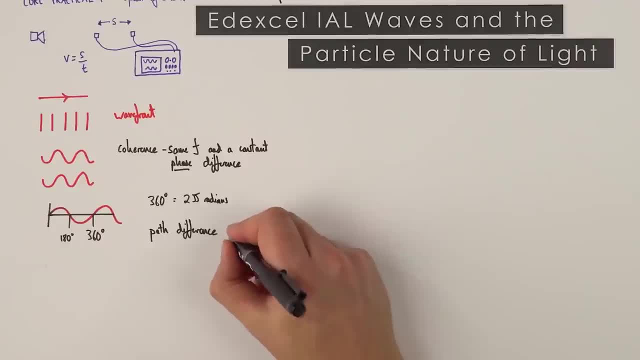 And the path difference is often given in multiples of the wavelength, but this is a distance and therefore it's going to be measured in metres, So we can maybe compare two different waves. They might have travelled a different length and that's our path difference. 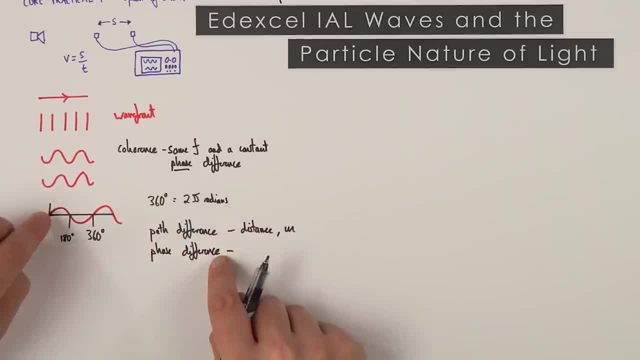 Whereas phase difference is really about the difference between which part of the wave cycle two waves are in, And because this is the phase difference, it's going to be an angle and then that's going to be measured in either degrees or radians. So they sound similar, but they're actually quite different. 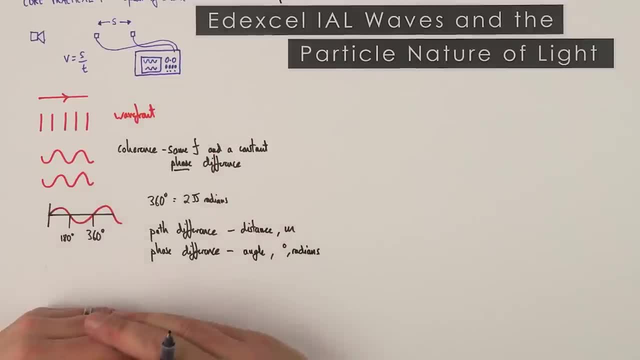 And this is important, because what we can have is one wave interfering with another wave, And this is where we have things like superposition And, effectively, what we can say is that we add up the individual displacements of those two waves to get the total displacement. 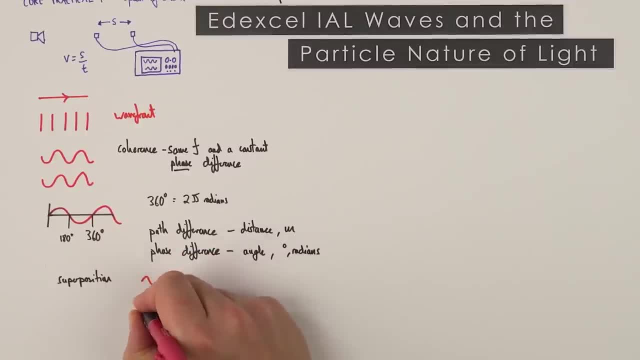 So, for example, if we had two waves which are in phase, that means that when you add the amplitude of these two waves which are in phase together, it's going to sum up to give something bigger than what we originally had. So you've got a maximum displacement here. 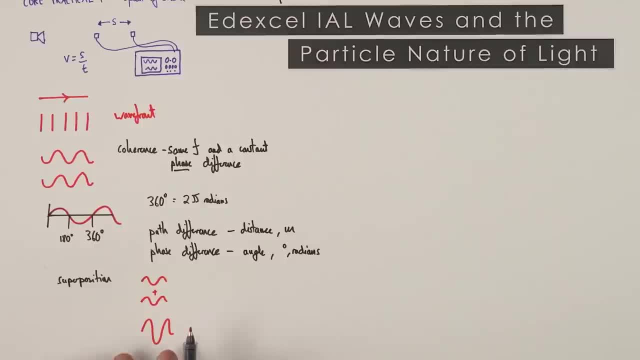 Maximum displacement here gives a massive maximum displacement when you have the superposition of two waves. If, however, you had waves which had a phase difference of 180 degrees or pi radians, then what's going to happen is that the peaks and troughs 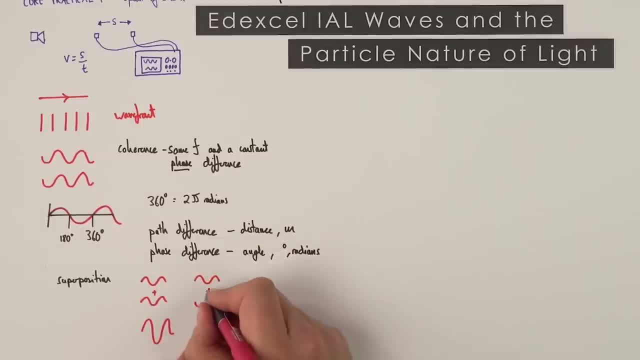 they're going to cancel with each other, And that means, if you added these two waves together, what we'd find is that the two waves cancel out and there's going to be no displacement. So this is because waves can interfere with one another. 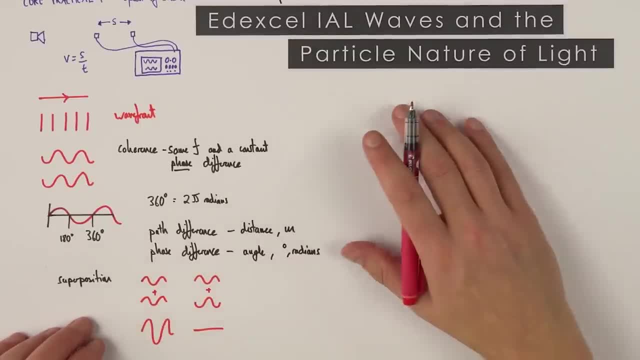 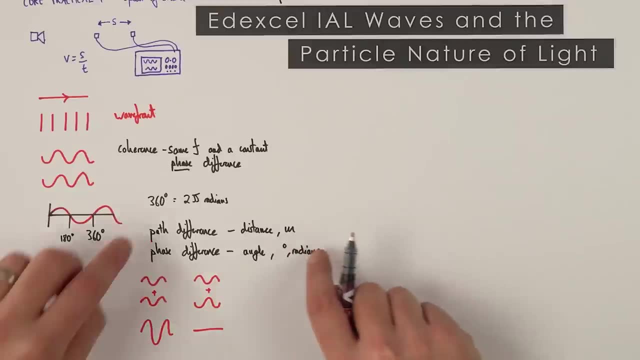 And again, this is quite important later on when we're going to be looking at the diffraction and interference patterns of waves. And, as a final thing, these two things are related because if you have something where the path difference was equal to lambda one wavelength, then the phase difference 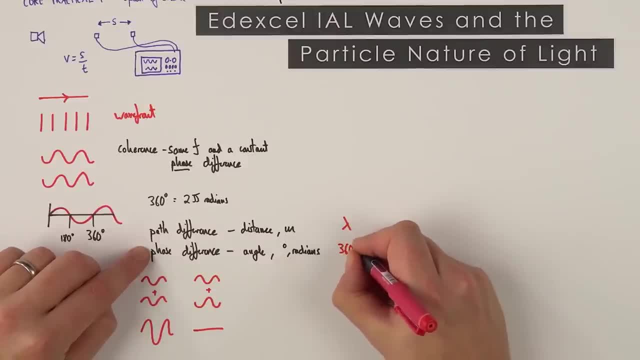 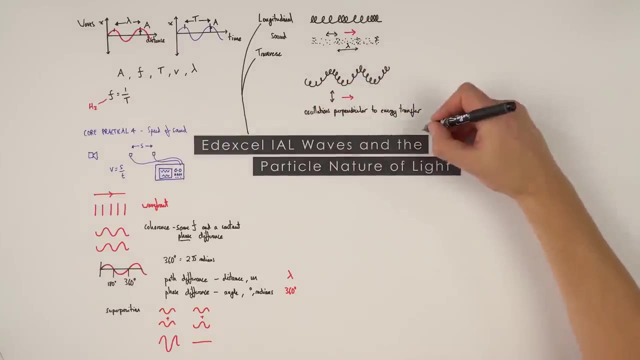 it's going to be equal to 360 degrees, or two pi radians. So there is a relationship between the path difference and the phase difference between two waves. Now, so far we have looked at progressive waves, which is transferring energy from one place to another. 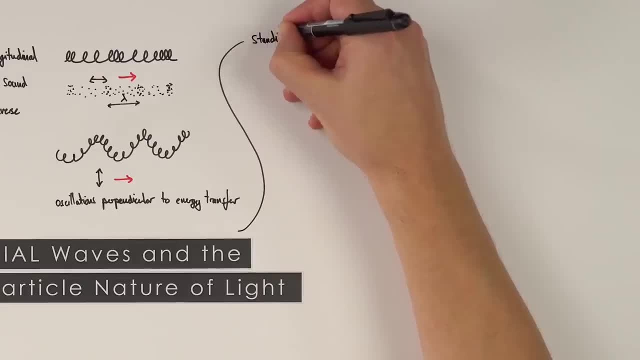 but there is another type of wave that we call a standing or a stationary wave, And what these do is they store energy. Now, effectively, if you had a wave like this and it was moving in one direction, it could reflect off something. 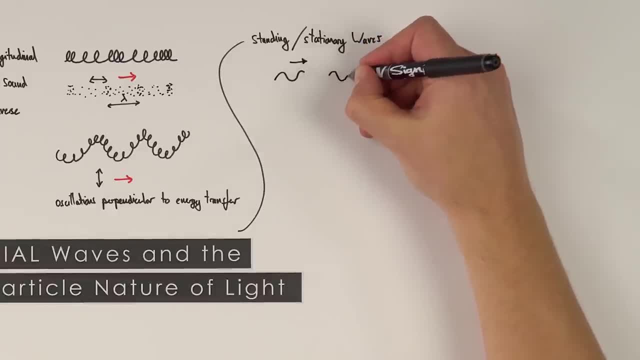 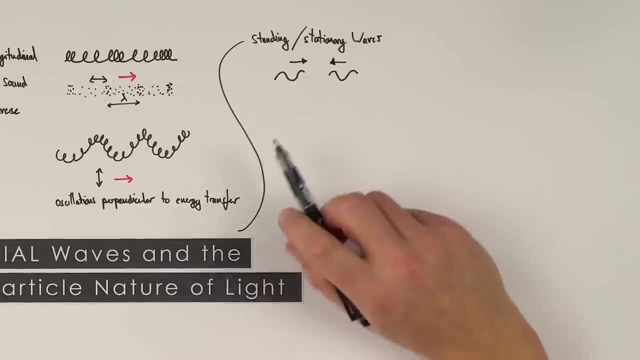 and then that wave would then travel back, And what you then have is two waves which are going to be coherent because they'll have the same frequency, They'll have a constant phase difference and a similar amplitude, And these two waves are then going to interfere. 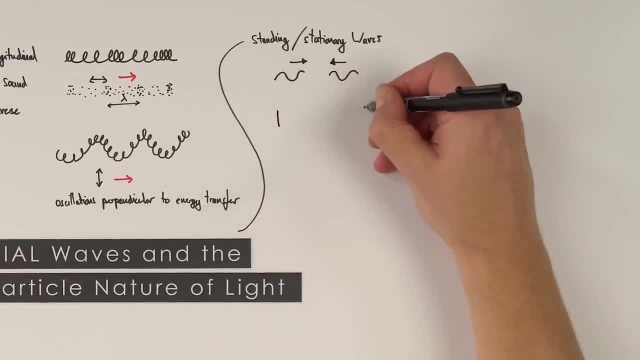 And the pattern that they produce. we can often demonstrate in the lab, perhaps using a string. Now I'm going to draw a couple of fixed ends over here. Now I'm going to draw a couple of fixed ends over here, And what we might see is a pattern. 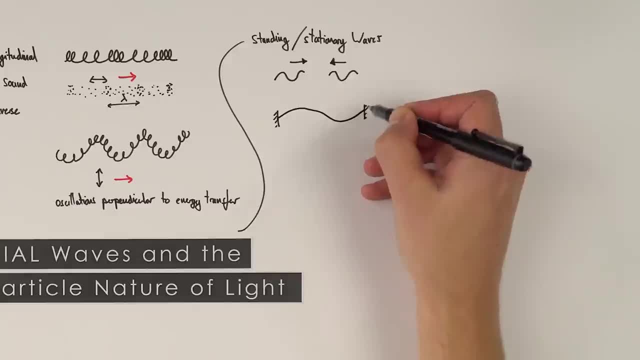 where the string goes up and down and back again. So that's one wavelength And then a short amount of time later it looks like this: Now, this is what we call a standing or a stationary wave. We have a position in the middle. 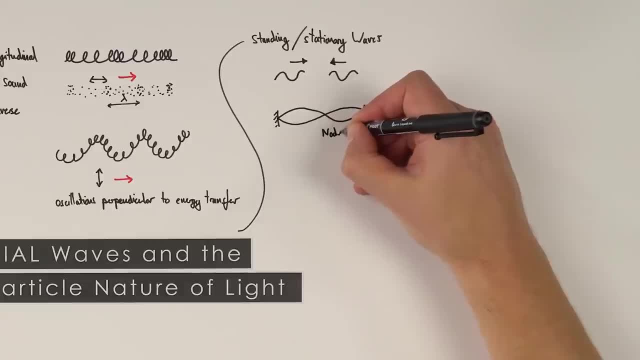 where there's no displacement, and this is what we call a node, And that's going to be at this time in the centre, And we also have these positions here where we have our maximum displacement, and that's the opposite to a node. 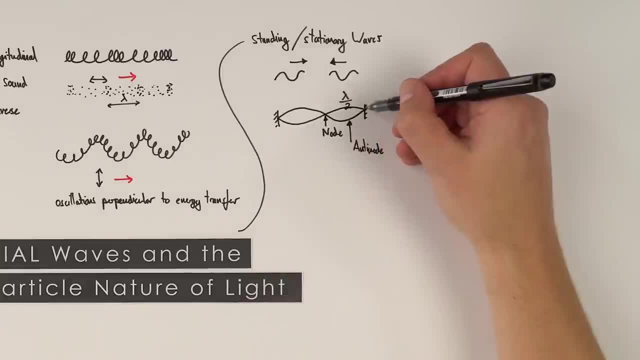 So that's going to be called our antinode, And here the distance between a node at the end and the node here is equal to half the wavelength, because one wavelength goes up, down and back up again. Now, this is just one of the possible ways. 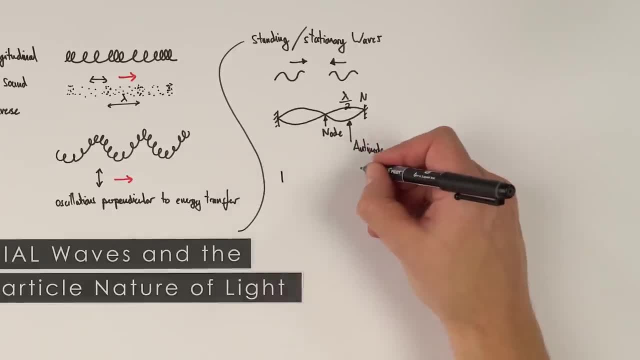 that perhaps that vibrating string could be The first one. it would be would actually just be having a node at each end, at these fixed ends and the antinode in the middle. So this is often what we call our first harmonic, And as we increase the frequency, 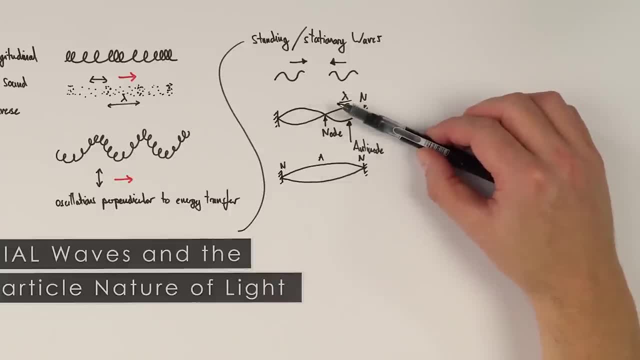 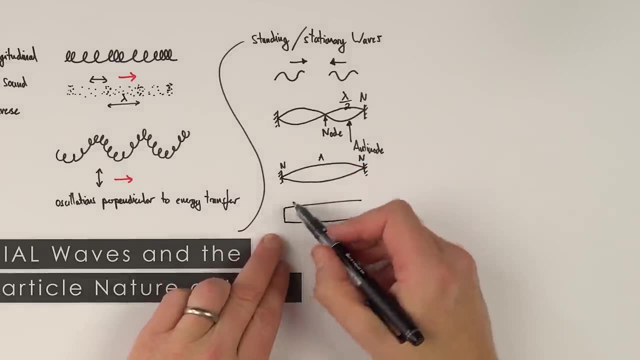 we get to other certain frequencies where we have these standing waves formed. We can also form them in a tube, and this is perhaps where we have some air which is oscillating. And here we've got our fixed end and the open end. 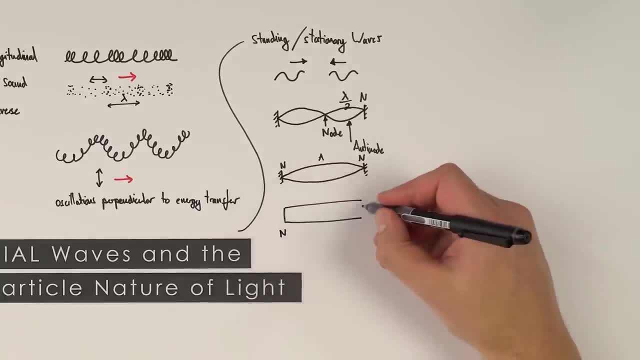 And what we find out is that the fixed end is where we have a node and that the open end is where we have an antinode. So, again, one of the possible things could be that, if you've got a node, maybe an antinode here. 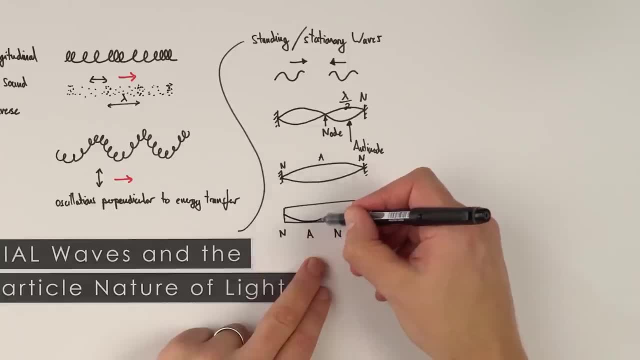 a node here and an antinode there, So we'd maybe get something that looks like this, And this picture here is really just sketching the maximum displacement of each part of that wave. Now, the other thing about these waves is that if you wanted to work out how quickly they're going, 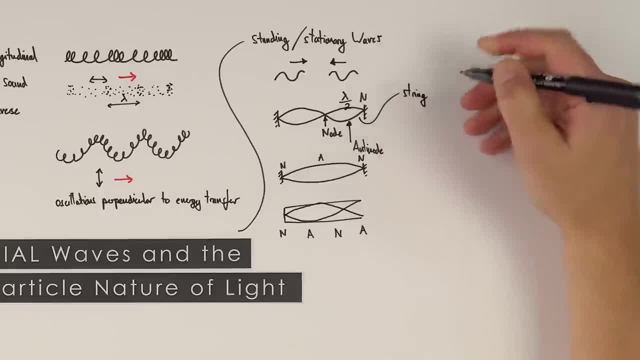 especially if you have a string, then the speed of that wave V is going to be equal to the square root root of t over mu. So here t is our tension in that string and here mu is what we call the mass per unit length. And this equation is really useful because there again is another core, practical. 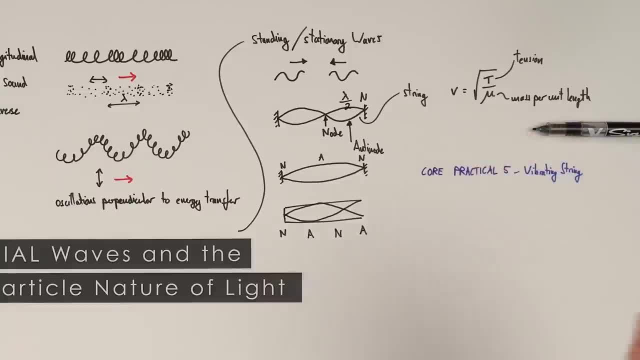 this time it's core, practical five, And what you can do is set up a vibrating string in the lab. Often this is done on top of a table. you have a vibration generator at one end, you maybe have a pulley at the other end, and this allows you to vary the tension in that string which runs over. 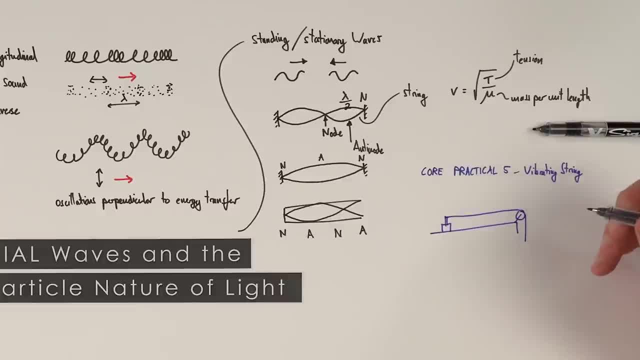 that pulley And what you can do is you can look at the things that affect the frequency. Now, the frequency is going to depend on certain things. It's going to depend upon the length of that string, the tension in the string and also the mass per unit length of that string as well, And all of 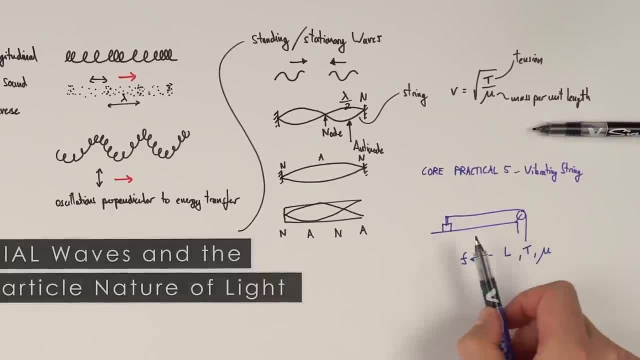 these are going to have an impact on the frequency where we have the standing waves formed. Now I've got an example of a standing wave and I've got an example of a standing wave and I've got an example of another video where I go into that in a bit more detail. But this is why you need to know. 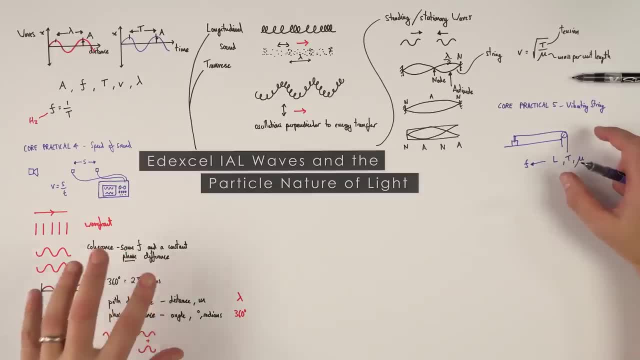 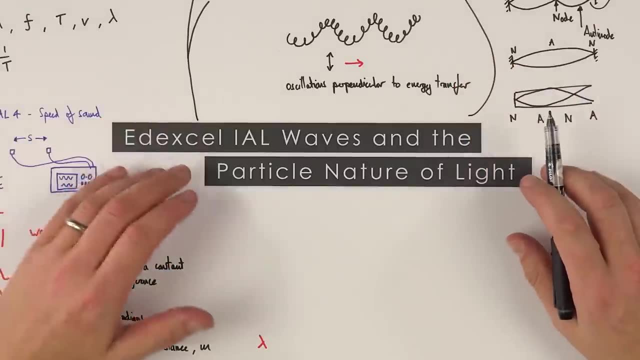 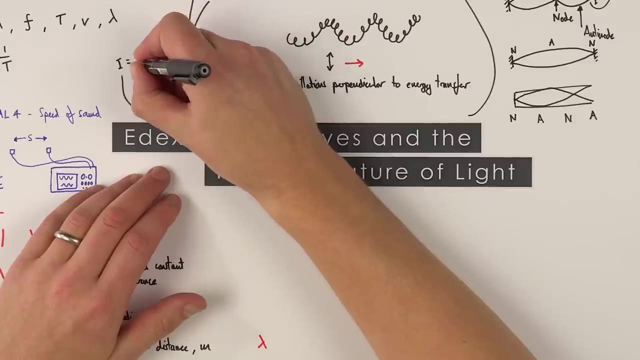 about how standing waves are formed by the interference of coherent waves. Often, when we're looking at waves because they're transferring energy from one place to another, we can actually look at the intensity I, which is actually equal to the power divided by the area. So this is the 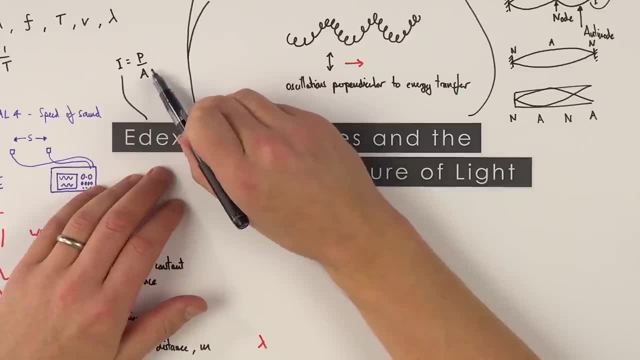 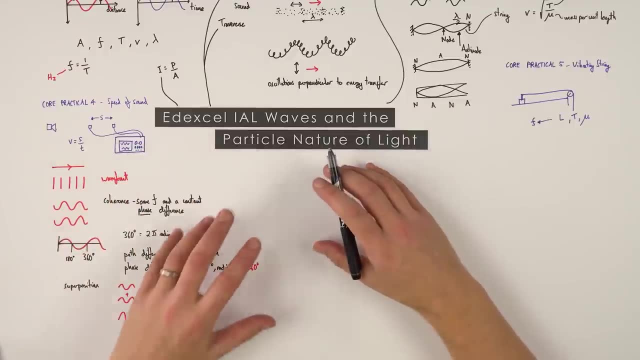 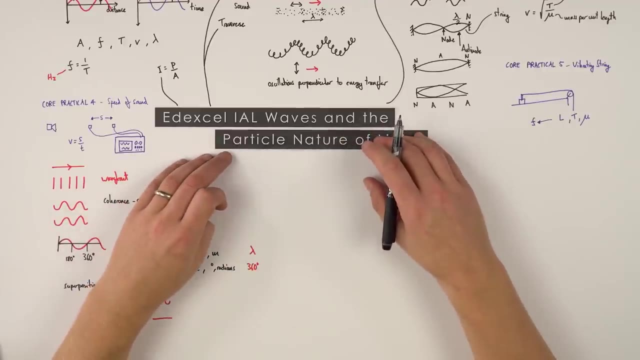 amount of energy transferred per second, and that's the area that that wave is instant on. So intensity is equal to power divided by area. Now, another thing we often tend to look at when we're investigating waves is the behaviour of light, in particular as part of the EM spectrum. 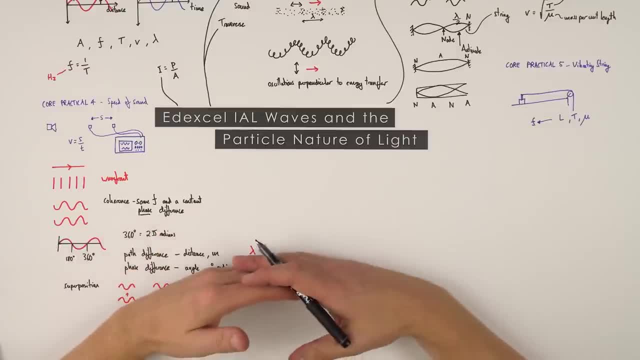 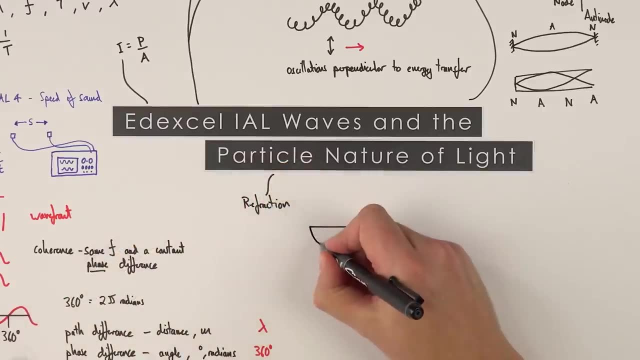 Now, one thing that light can do is as it goes from one medium to another, it can actually change direction and we call this refraction. Now the standard school. practical is that you maybe have a perspex block. I'm going to call that medium. two, and I'm going to call that. 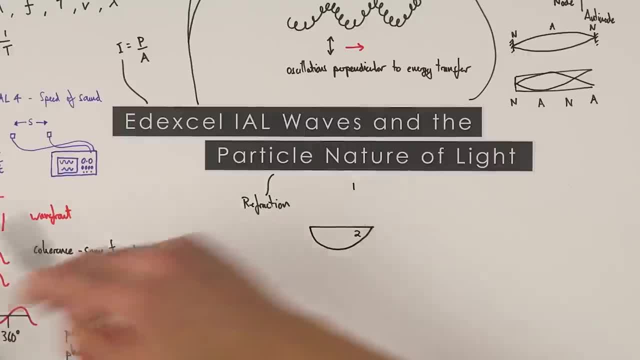 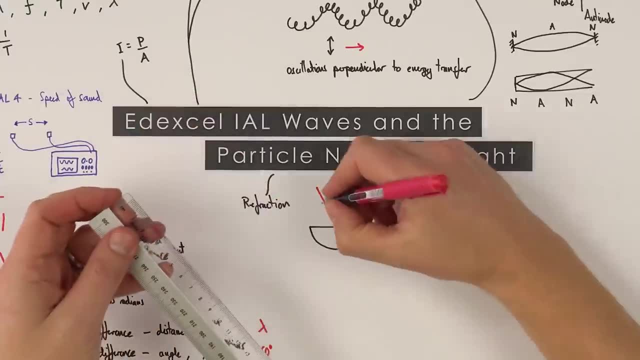 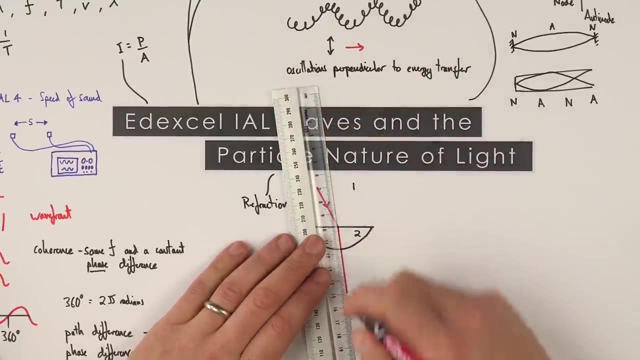 air medium one. And if we were to shine a ray of light, I'm just going to draw it here, using a ray to represent the direction that it's travelling in. As this ray of light meets this block, it changes direction, And the reason for this is that the speed of light, or the speed of this wave in 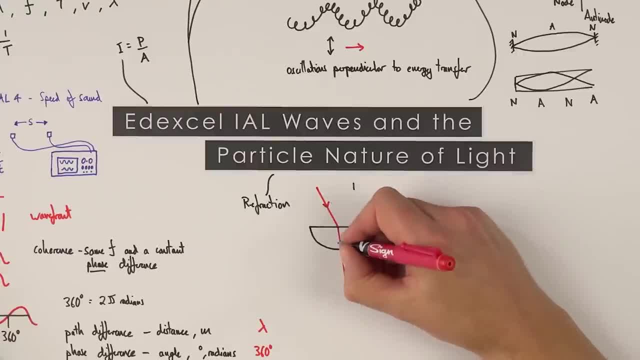 this medium is different to the speed in this medium. So what happens is it goes through the block and then it keeps going, because it meets this at a medium. So if we were to draw a ray of light at 90 degrees, it keeps going in a straight line. Now, here again, this should be a revision of 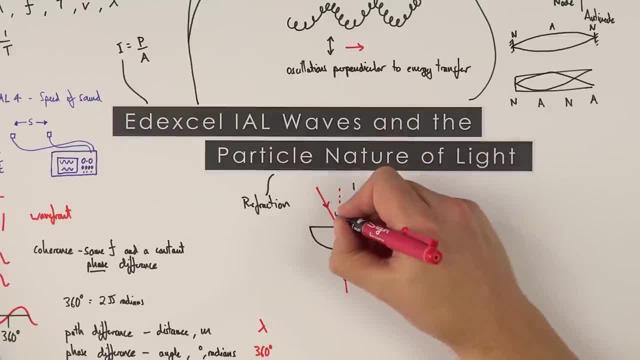 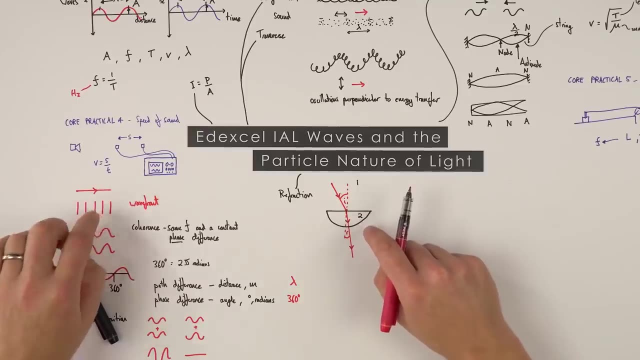 what you've covered before A-levels is we have the angle of incidence and the angle of refraction R. Now why does that happen? Well, the reason it happens is often explained better by considering the wavefront way to actually represent waves. So if I was to maybe draw this boundary close up, 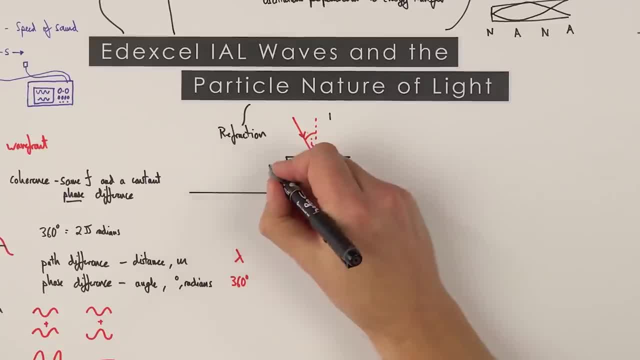 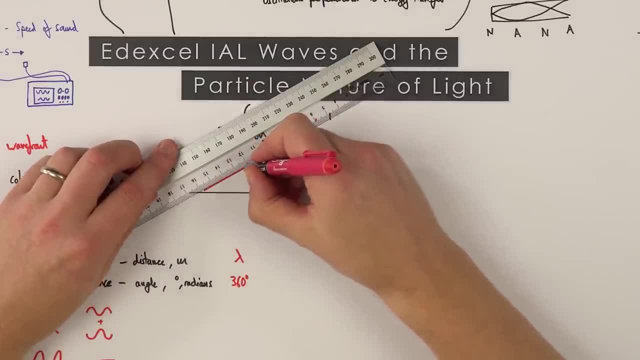 like this: we have a ray of light, and then we have a ray of light, and then we have a ray of light and then we have medium one here and medium two, Even though the wave is travelling in this direction, we can consider the wavefronts of light as they approach that surface. And if we 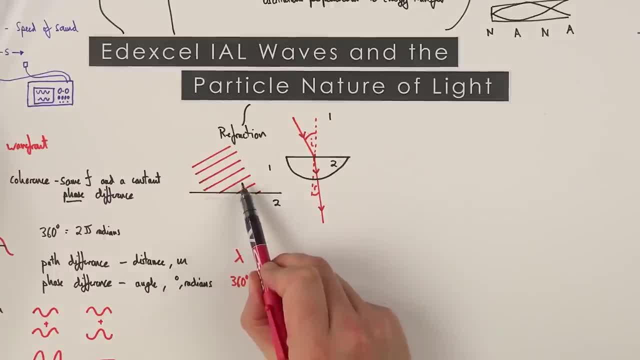 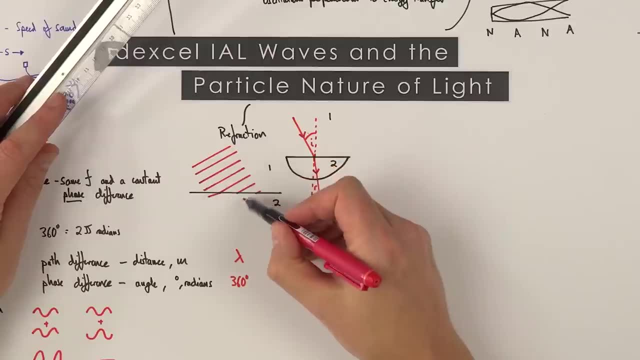 consider this wavefront here, some of it's going to meet medium two before the other bit, and that means it's going to slow down first And as it slows down it changes direction. And the same for this one over here, because some of that wavefront meets the surface before the rest of it. 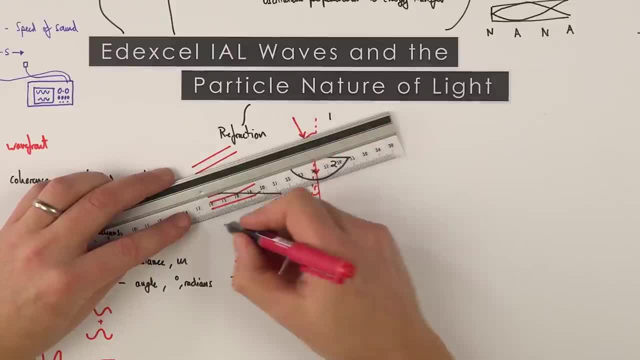 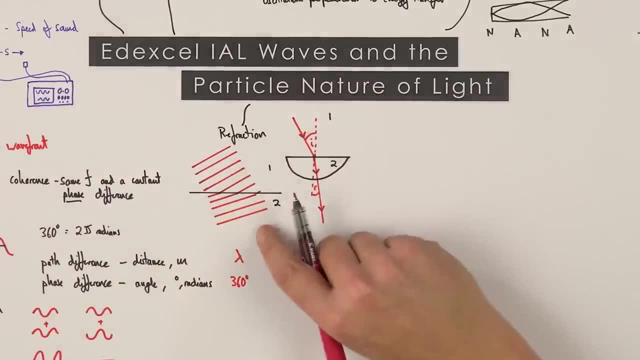 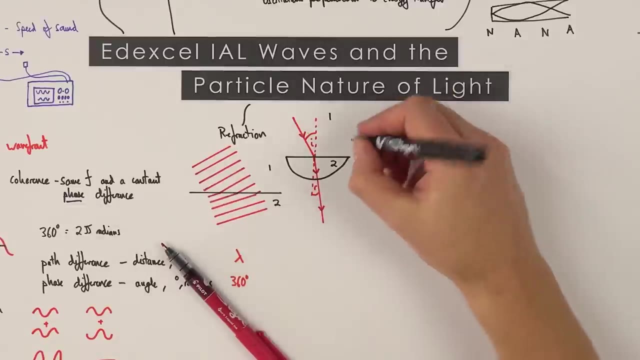 slows down first, And then, as it goes through the medium, it's all travelling at the same speed, so there's no change in direction. We only have the change in direction at the boundary. Now, like all things in physics, there's going to be an equation that actually explains this. 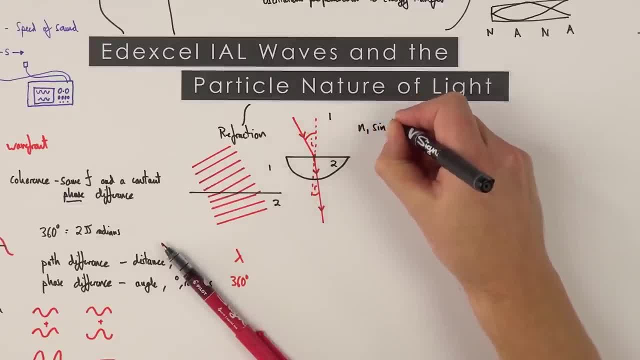 and what we can say is that N1 sine theta 1 is equal to N2 sine theta 2.. So here N1 and N2 are the refractive indexes of medium one and two, and here this is going to be theta one and this is 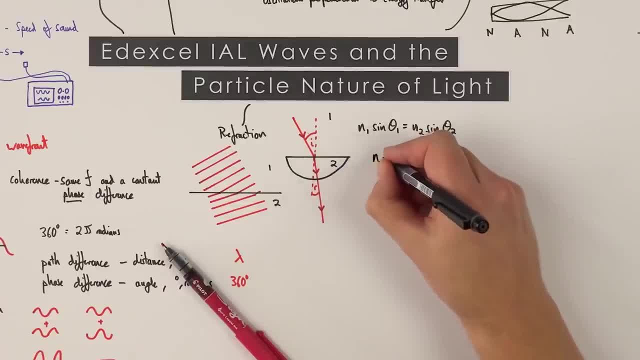 going to be theta two, And the refractive index N is equal to the speed of light divided by the speed of light in that material, And this basically tells us by what factor the light slows down. And it's going to depend if you have glass or diamond or perspex. 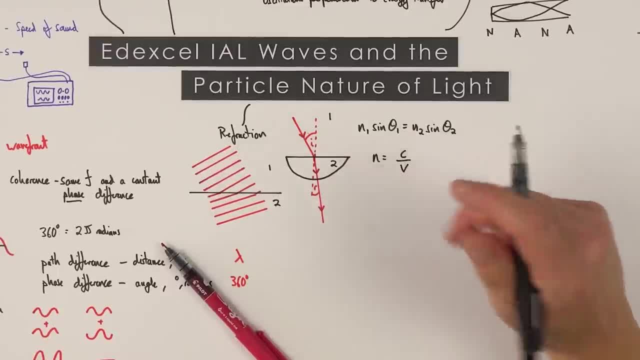 different materials slow down that light by a different amount, And because it's the ratio of two speeds, it has no units, And if you wanted to measure this refractive index in the lab, what you could do is an experiment a bit like this, using some light. If you've got values for 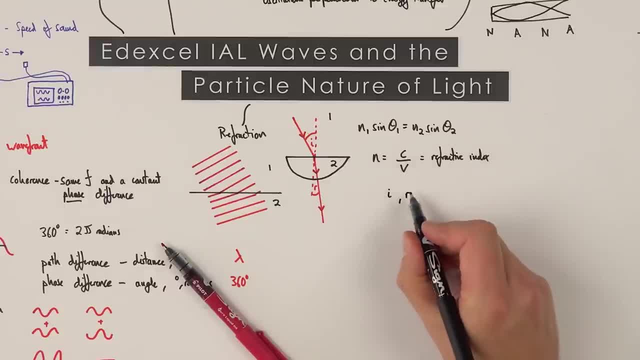 the angle of incidence i and the angle of refraction r. what you could then say is that the refractive index is going to be equal to sine i divided by sine r. But you'd do that not just with one data point, but you'd maybe look at many values of i. 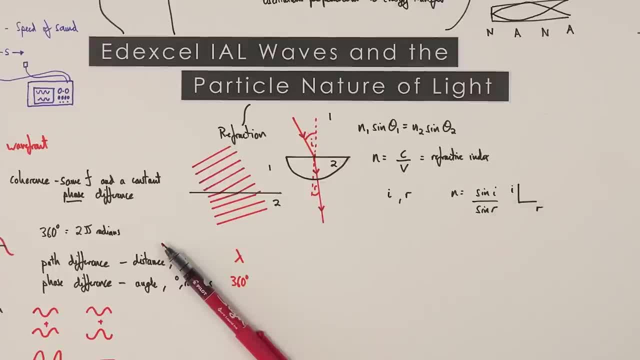 And many values of r. You could plot this on a graph and actually work out the gradient of sine i and sine r. So that's the way that you could actually measure this yourself in the lab. Now this is a little bit more interesting when we actually think about not light going from. 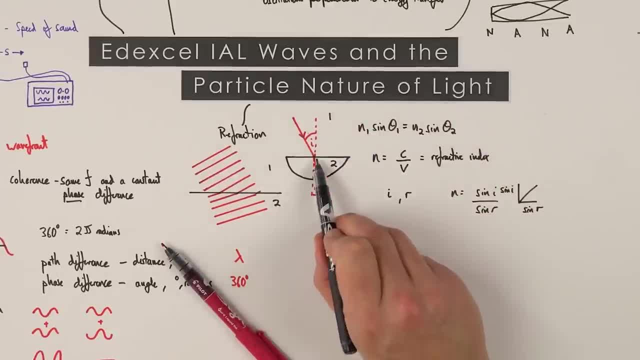 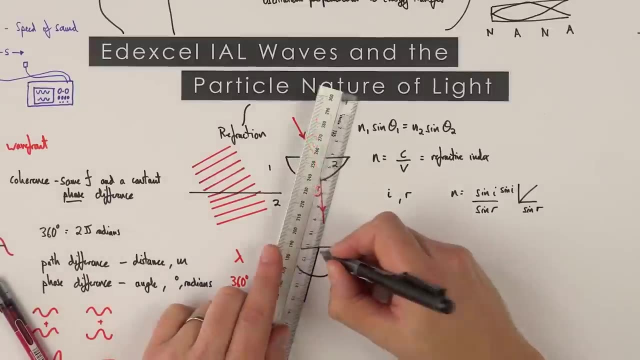 maybe air to glass, but maybe the light going from the glass back into the air. Now I'm just going to draw this same perspex block one more time. So just a quick sketch. Now, if we sent a ray of light potentially like this, and so here is my normal line, drawn at 90 degrees. 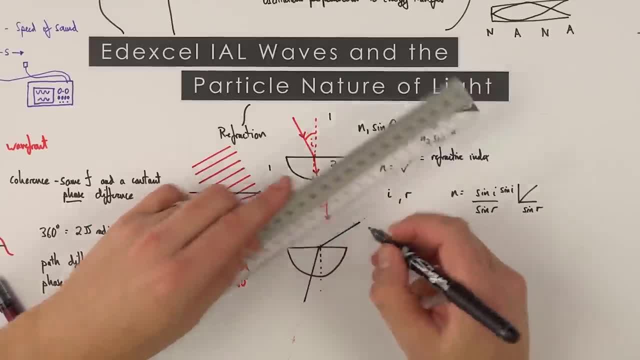 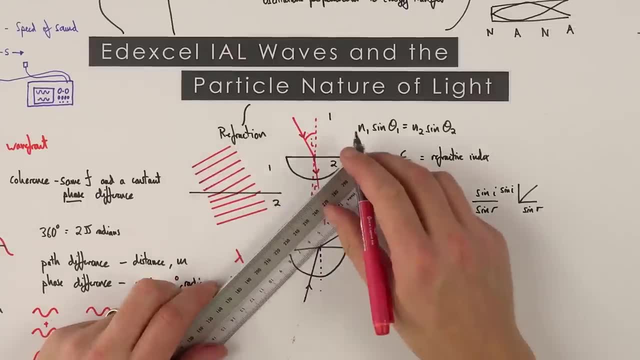 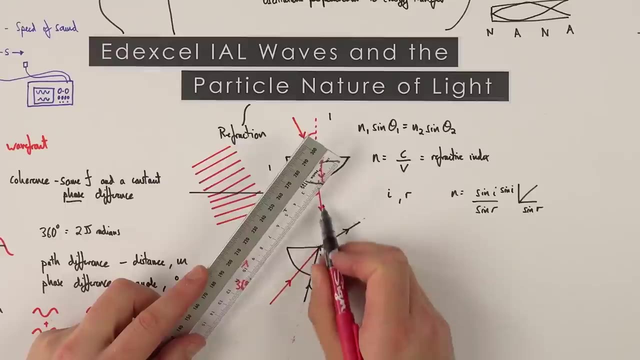 to the surface, some of that light is going to escape. But if I was to increase the angle of incidence here, we're going to get to a point where the angle of refraction is equal to 90 degrees. So at some critical angle, even though the light comes in, none of that's going to be. 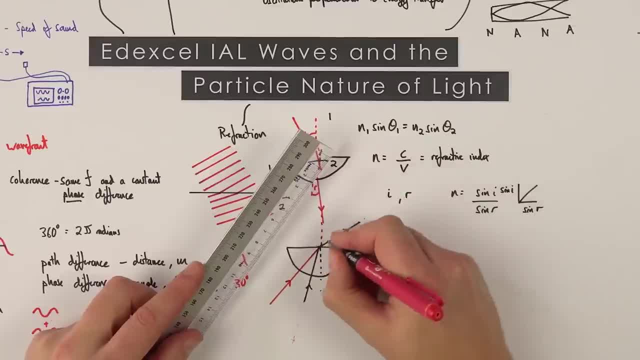 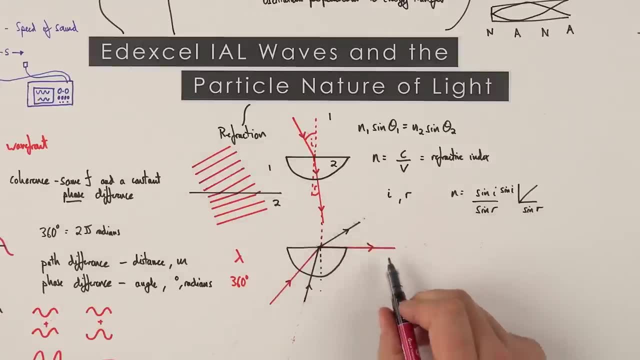 escaping out in this direction, because this angle here, the angle of refraction, is going to be equal to 90.. And if I just continue that ray of light, what happens at this particular angle is that all of that light travels along the boundary of these. 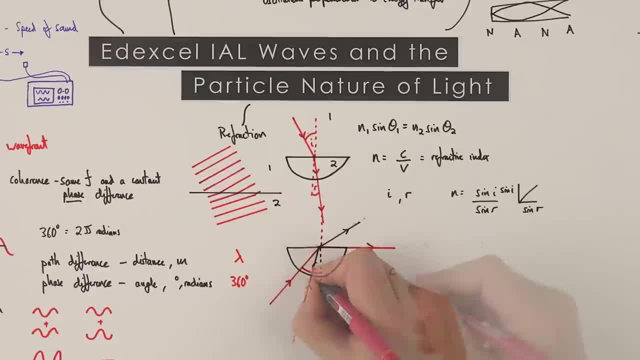 two things, And here this angle c, this is what we call the critical angle, And what we can say is that 1 over n is equal to sine c. So sine of the critical angle is equal to 1 over the refractive. 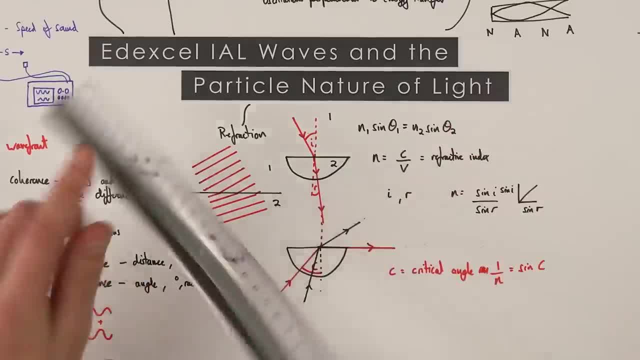 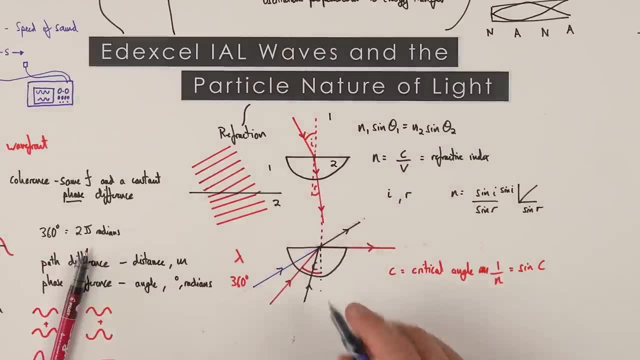 index. Now, if a ray of light was meeting the angle of refraction and the angle of refraction was meeting this particular point at an angle greater than the critical angle, like this ray of light here, none of it would be escaping and, in actual fact, all of this light would be. 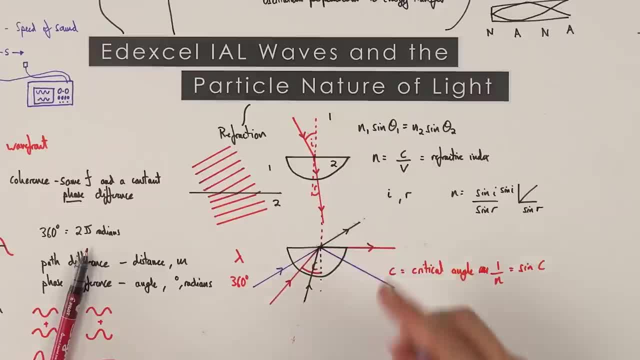 reflected off that internal wall. So here in blue what we have is something called total internal reflection, And this is when the angle of incidence is greater than the critical angle. Excuse all of the smudges here from the ruler. So what we have is, if you have light maybe travelling from an optically denser medium to a 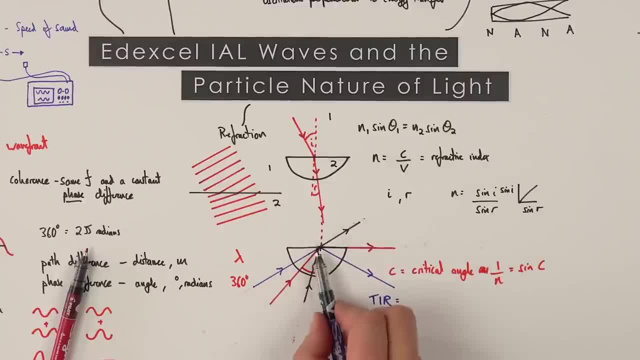 less dense, optically dense, medium, then at a critical angle. none of the light escapes and it's an angle greater than the critical angle. we have total internal reflection of that light. So you can see, we're using lots of different diagrams and models to actually represent what's. 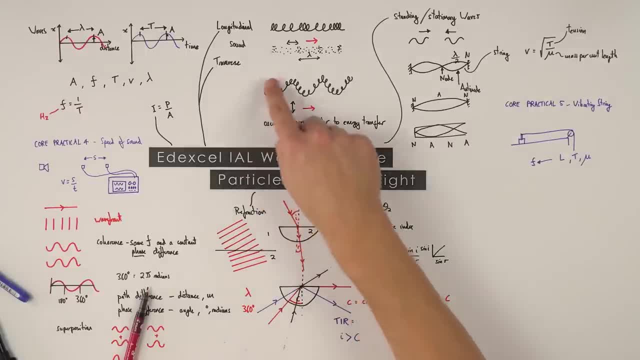 going on with the light. Now, if we consider a transverse wave, we've seen a side view of how the oscillations which are perpendicular to the light are reflected off the light. So you can see, we're using lots of different diagrams and models to actually represent what's going on with the light. 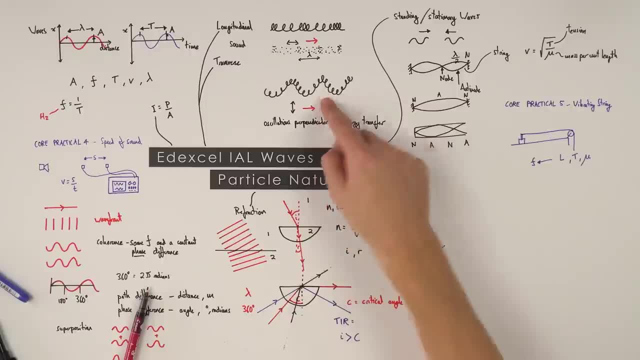 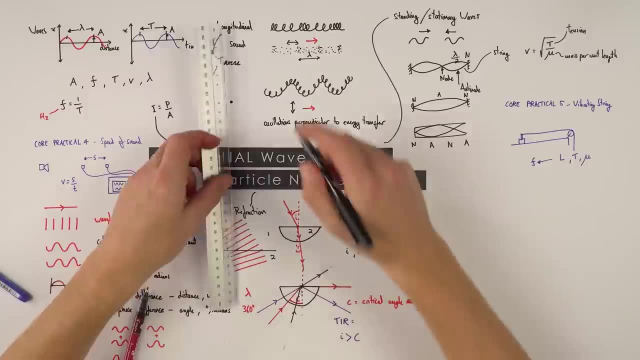 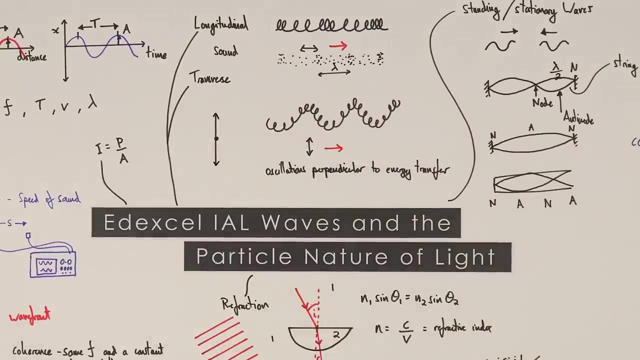 perpendicular to the energy transfer can be displayed. But if we were to imagine looking at this head on, what we might see is that if this is the wave coming towards us, we have oscillations, perhaps in this plane. So that's going up and down. Now, if you have something, 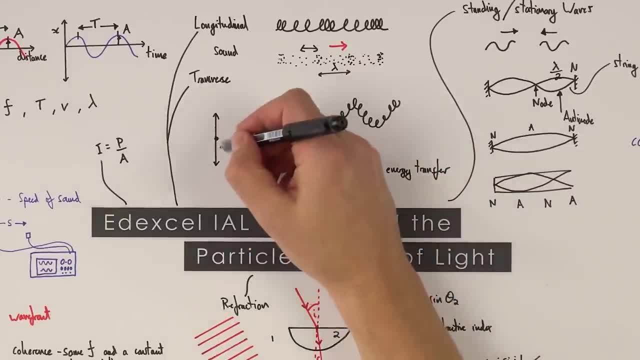 like an electromagnetic wave. for example, not all the oscillations are going to be up and down. some of them might be side to side, and then some of them might be at all sorts of different angles. So I'm just going to represent all of the different planes of oscillation like this. So this is what we call. 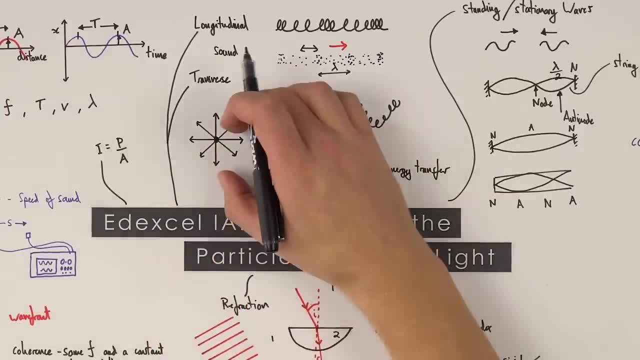 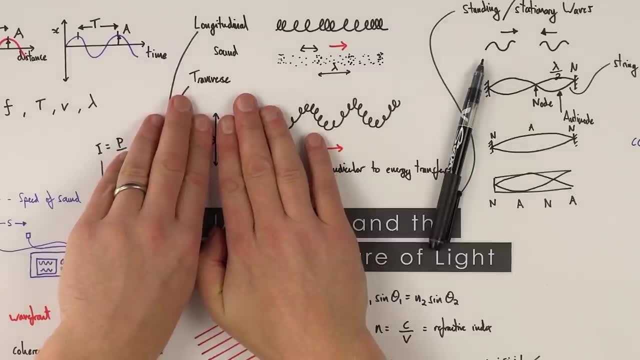 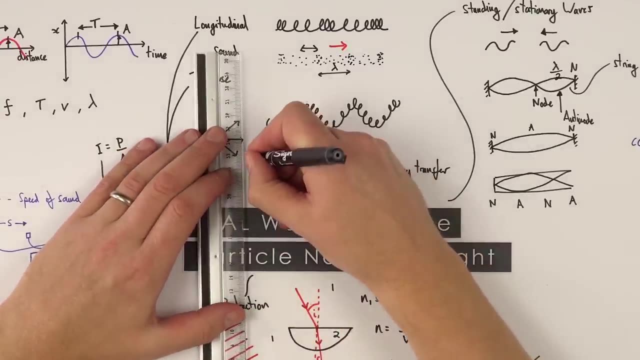 unpolarised light. But what we can do is we could pass this through a filter, and then what that would do is it would start to filter out all of the oscillations apart from those in one plane. And if you pass this light through that filter, what we'd find is that all of the oscillations 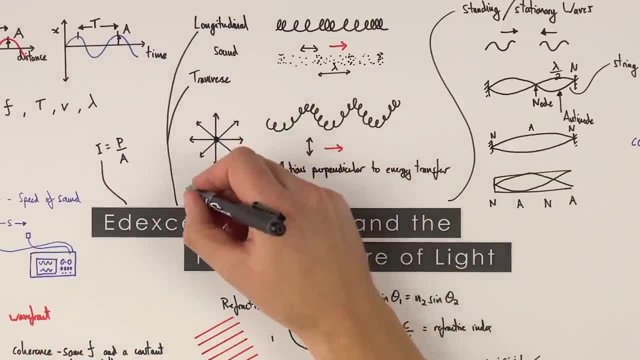 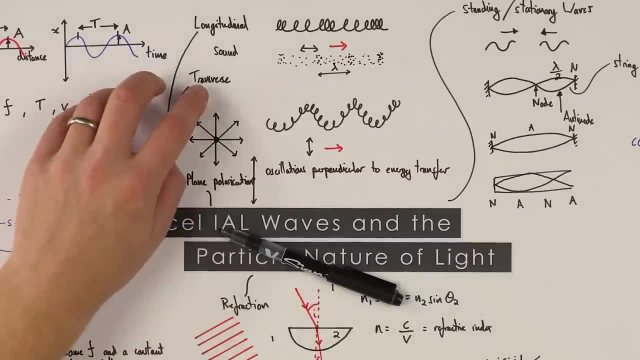 are in the same plane And we call this polarisation and this would now be a polarised wave. So this plane polarisation only occurs with transverse waves because they're oscillating at 90 degrees to the direction of energy transfer. We can actually show it with a couple of filters. 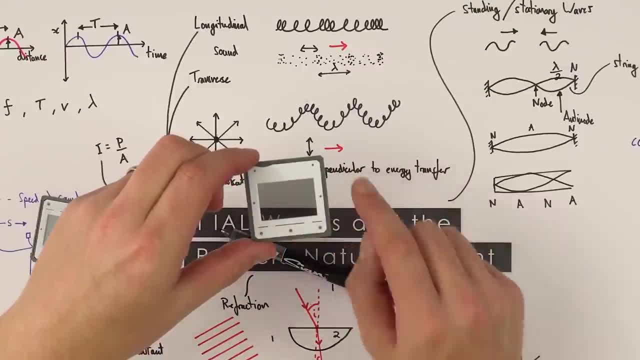 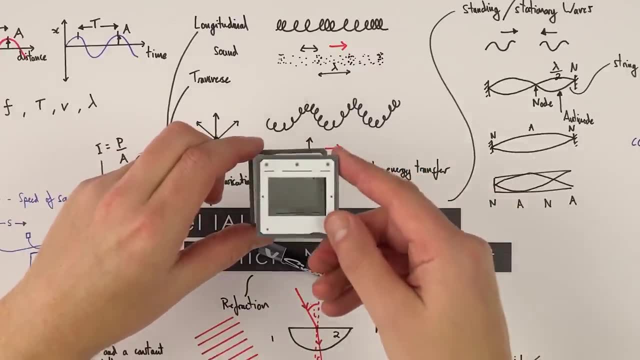 If I have just one filter, all of the light coming through this is now going to be plane polarised in the same orientation. If I have another filter that I hold in front of it, all of that light is going to continue to oscillate. 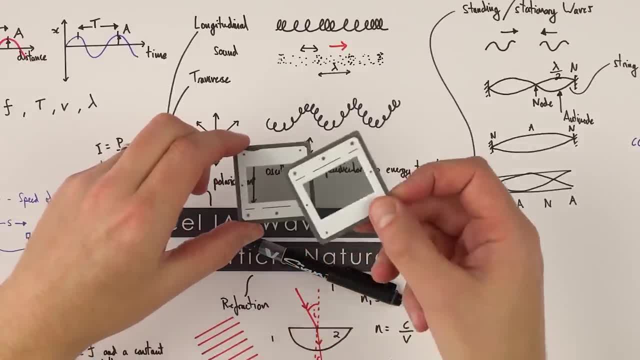 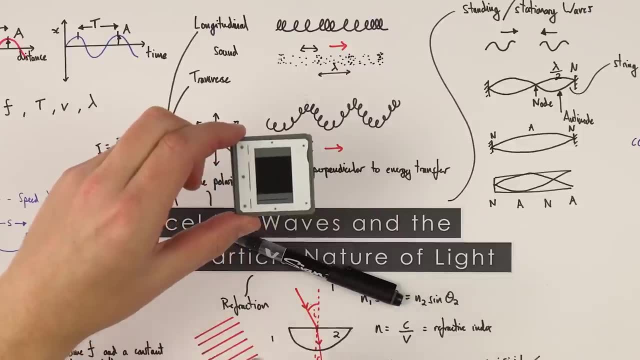 It's going to continue to go through both filters. But if I was to turn this filter through 90 degrees, what we can see is that now stops all of the light coming through, because we're cutting out all of the oscillations in this direction and also this direction. 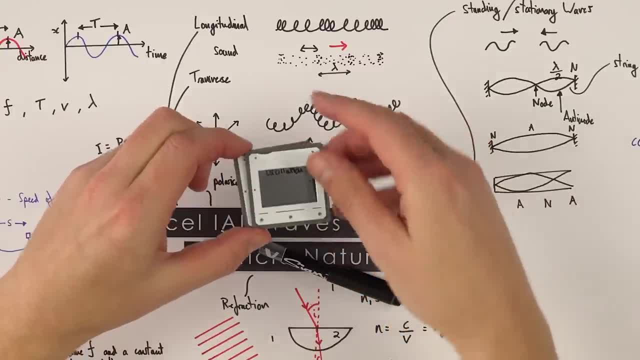 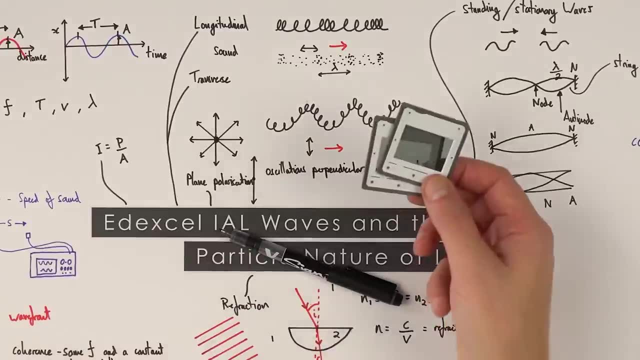 as well, Whereas if I rotate the filter around we can see that then lets that plane polarised light through yet again. So plane polarisation only occurs with transverse waves. It can occur with light, but also things like microwaves and other parts of the EM spectrum. 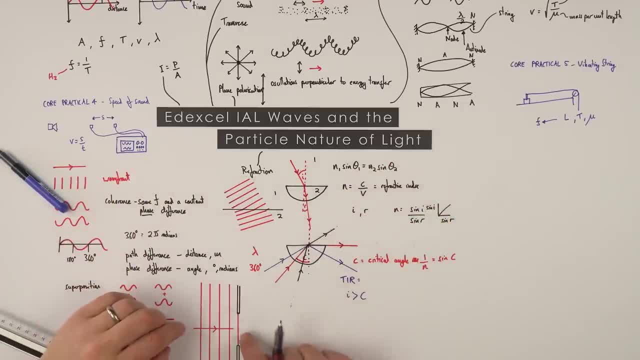 Now, if we look at this filter, we can see that this is a plane polarised light. Now, something else with waves, including light, is that when they meet an obstruction or a gap, what they do is that, as they go through that gap, they start to spread out. 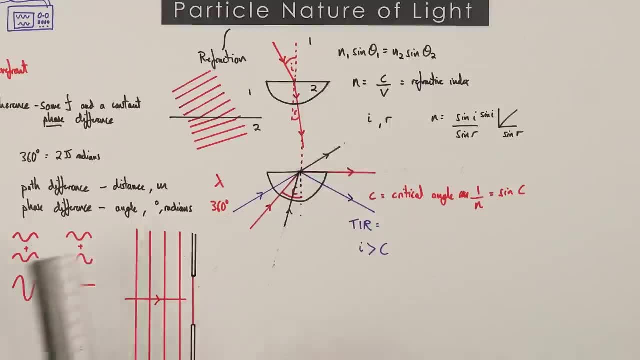 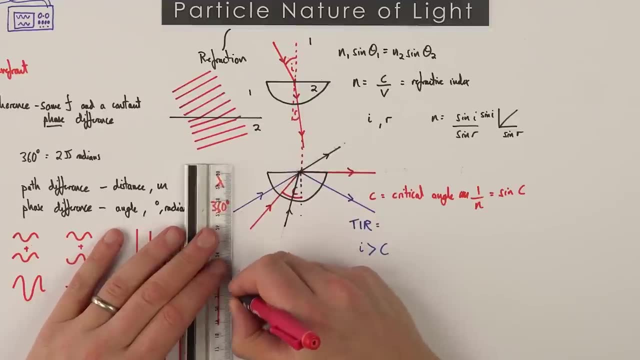 And here I've got the wave fronts, and this arrow just shows the direction that they're moving in. Now, here we've got a gap, And as the waves go through, the ones in the middle are going to keep going in the same direction, with the same wavelength, But they start to 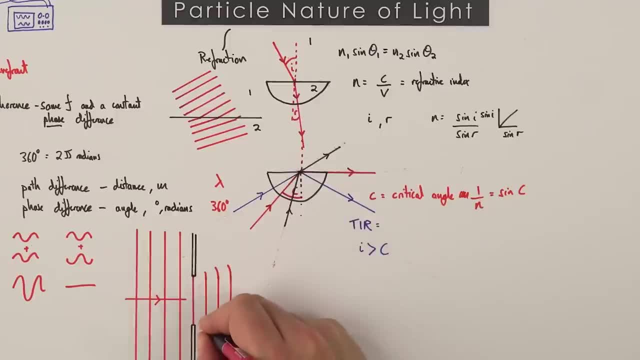 spread out a little bit around the edges, And this is the effect of difference. Now, what we find is that if the wavelength is approximately equal to the gap, that's when we have our maximum diffraction, And I'm just going to draw this with these semicircles. 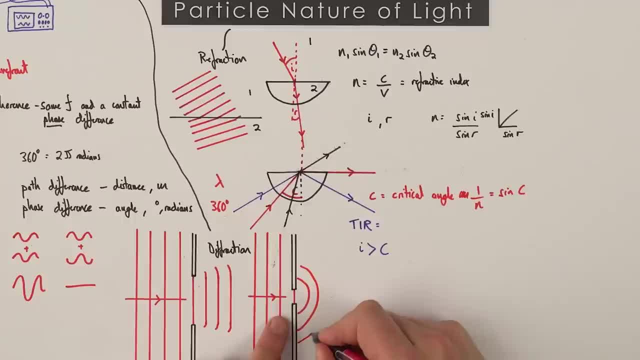 here, trying to keep the same wavelength approximately each time. So what we have is, when you have the gap equal to the wavelength, some of the light is going to- in this case, light, or it could be any type of wave- is going to go straight through and the rest- 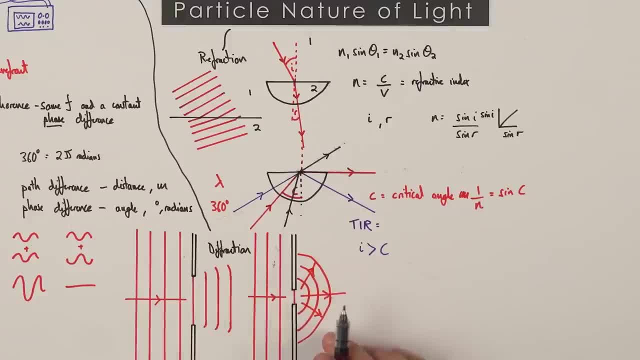 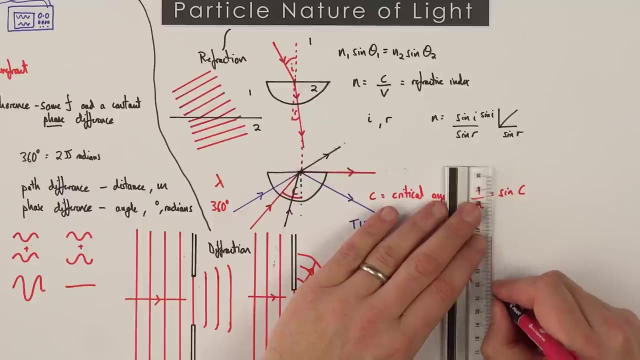 of it spreads out. Now, that's quite important. We're going to be looking at diffraction gratings in a minute. But why does it do it? Well, we can actually use something called Huygens construction, And this is a model that basically says how the next wave knows where it's going to be. 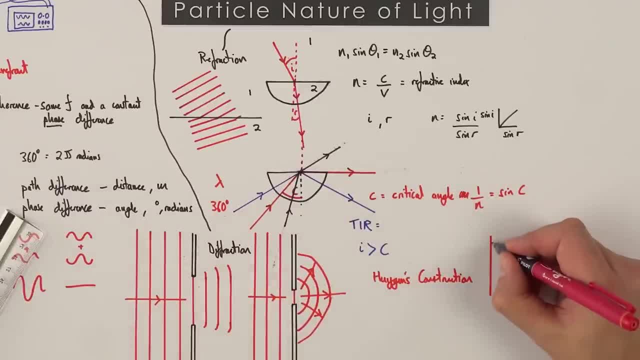 So perhaps we have a wave front here. What we can consider are multiple points along that wave front And effectively this is now another source of waves, And what we have are these waves spread out. Let's do the ones from this point over here And where all of these waves effectively join. 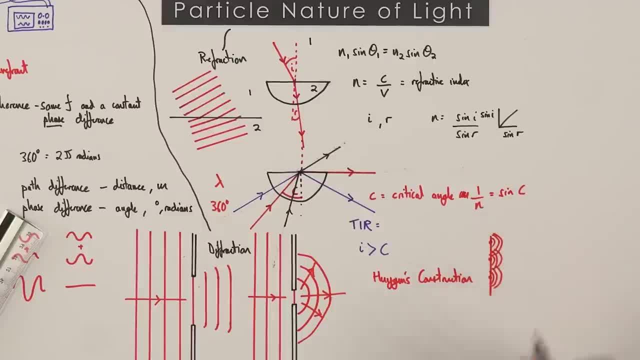 up again and interfere with this constructive interference is where the next wave front is going to be formed. In this case, it's going to be over here. Now, let's imagine that this was near a gap, So perhaps that's the edge of an obstacle. 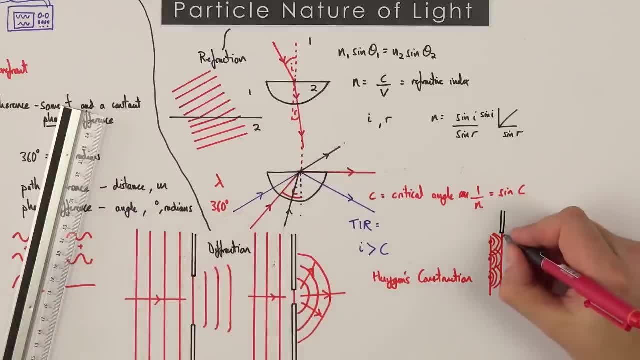 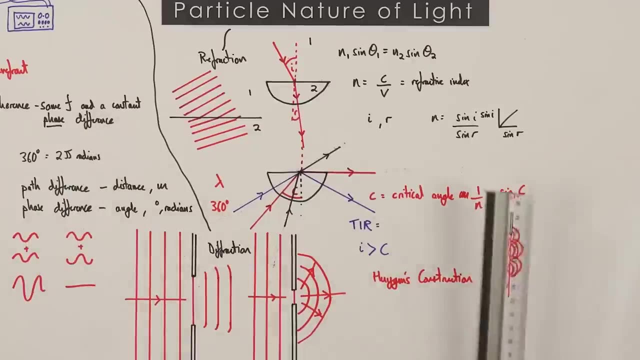 like we had over here. Well, from this point, this is going to be our source of secondary wavelets, So that's going to spread out like that. From here, we're going to have more spreading out like this, and so on. You get the rough idea. Now, if we were to join all of these points. 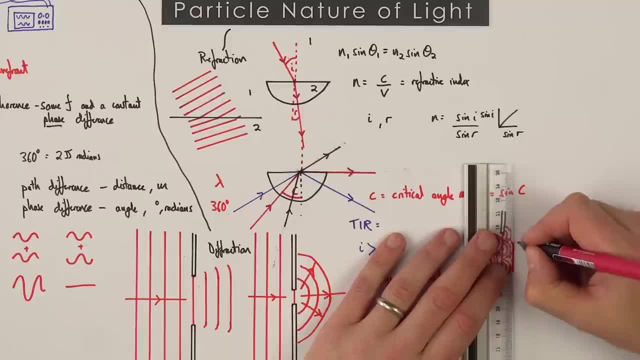 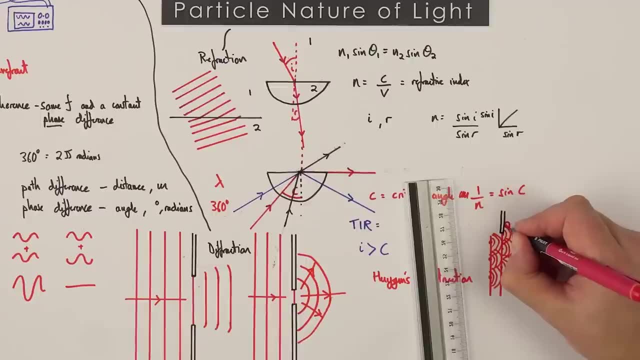 together. what we'd find is that these ones would be in that kind of straight line and around here that would move around the corner, And then from this particular point here we then have more wavelets and so on. Now it gets a bit confusing, but effectively what this is hopefully showing is that a wave. 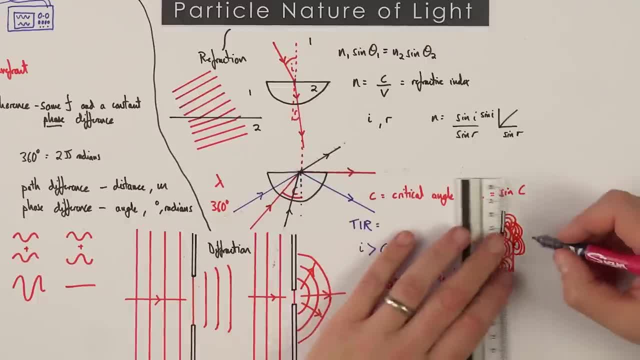 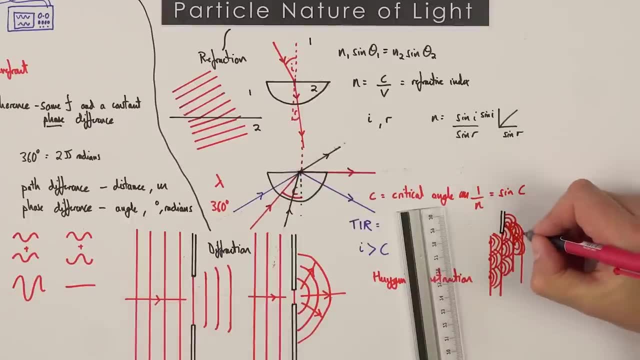 spread around the edge of an obstruction And if we were to again follow this on, we would have the main part of the wave moving through the centre of the gap and at the edges is where it starts to spread out. So Huygens construction- this is a model to explain how light behaves. 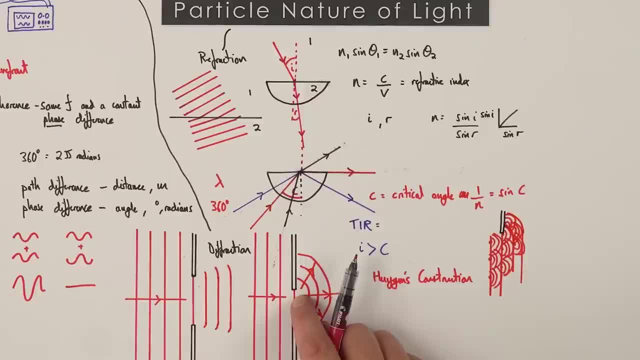 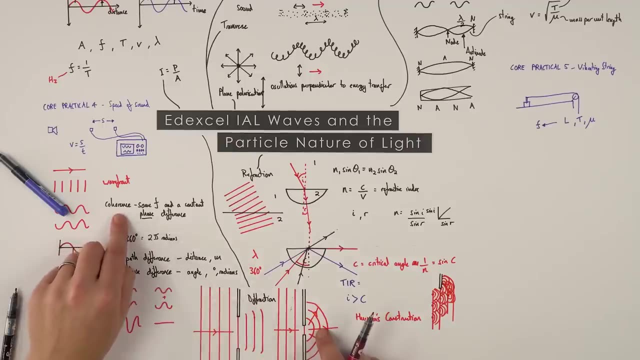 like it does when it gets to an obstruction like this. Now, if you had potentially multiple gaps here, what we'd find is that some waves spread out from this point, some waves spread out from the point next to it, and then we'd have interference of coherent waves. We'd have 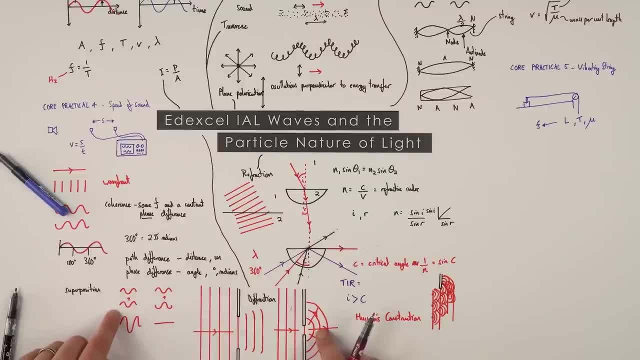 positions where the wave might constructively interfere and also destructively interfere, And a great example of this is something called the diffraction grating. Now, if you were to zoom in on the diffraction grating, you'd see multiple slits where the light can come through, And this 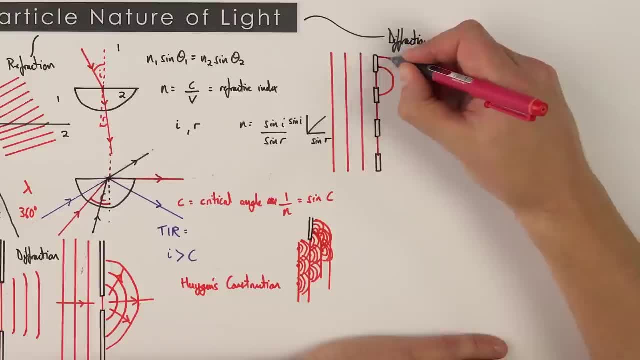 one. here there's going to be diffraction and this starts to spread out like so, And the same happens at this point, And if you were to zoom in on the diffraction grating, you'd see multiple slits where the light can come through, And this position, and this position and so on. Now, as the 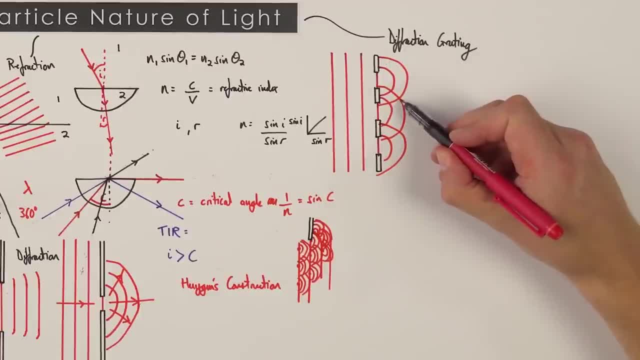 light continues to move forward. there's going to be points here which are in phase and therefore we're going to have constructive interference, perhaps where a peak adds to another peak. There's also going to be positions where we have destructive interference, where the waves 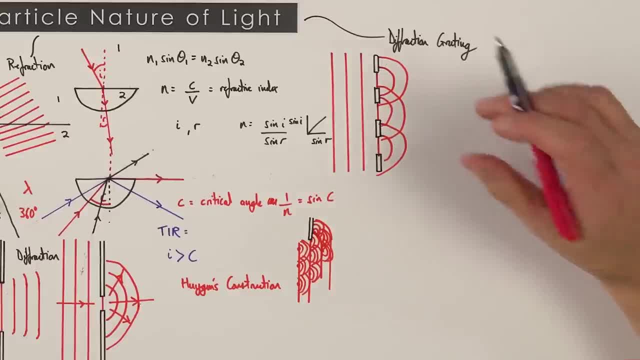 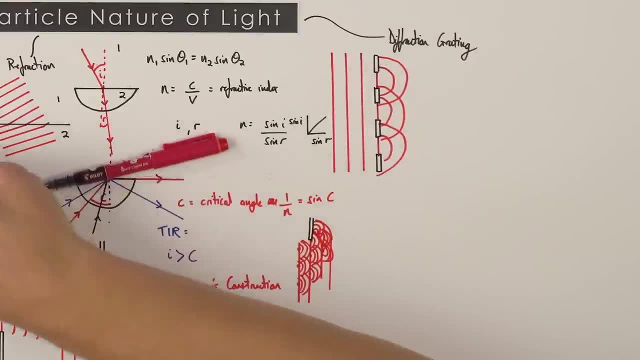 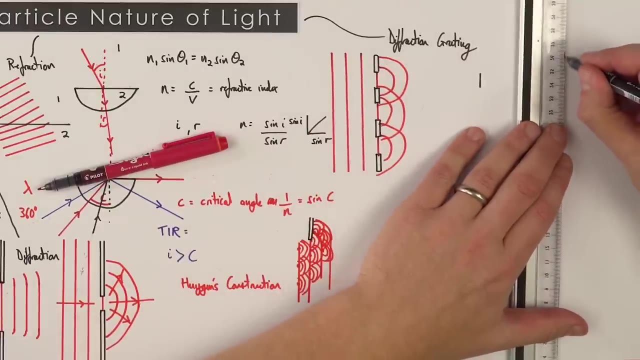 are perfectly out of phase. So that's a phase difference of 180 degrees or pi radians, and here we're going to have destructive interference. Now, to sort of zoom out of this, perhaps this is my diffraction grating and this is a screen which 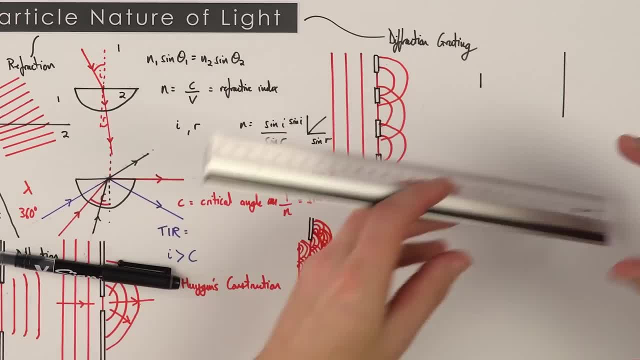 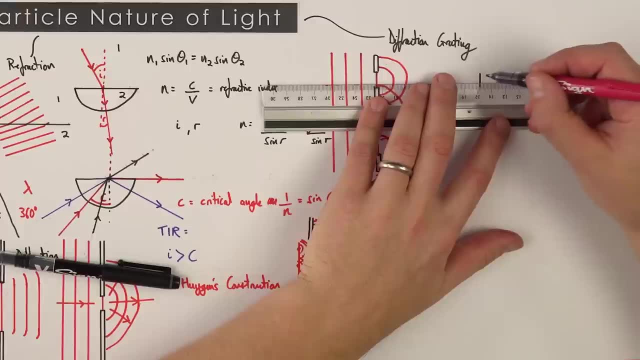 might be several metres away If we were to shine laser light as an example. because laser light is coherent, it's all exactly the same wavelength and therefore same frequency. some of that light is going to go through the diffraction grating, it's going to hit the screen and at the middle, 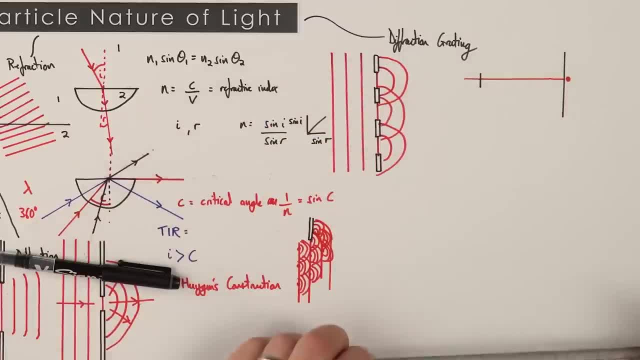 here we're going to have a bright spot that we observe. There's going to be other points where there's going to be destructive interference, and then, a small distance away, there might be another bright spot on each side, and then another bright spot, and so on, And what we 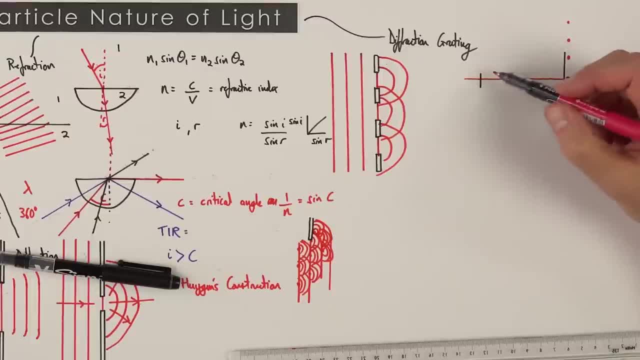 see are a series of bright spots, especially if you're using laser light with a diffraction grating. Now this one here is the zeroth order. this is our first order, and then we've got our second order, third order, and so on. 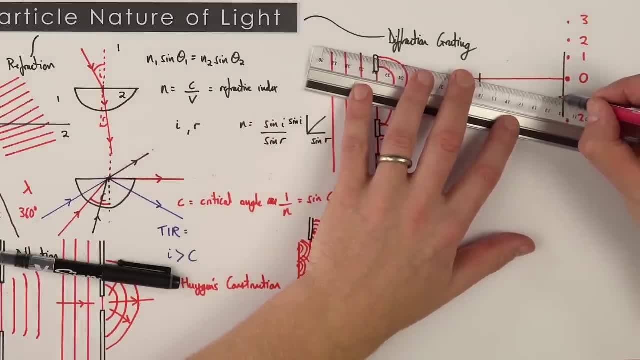 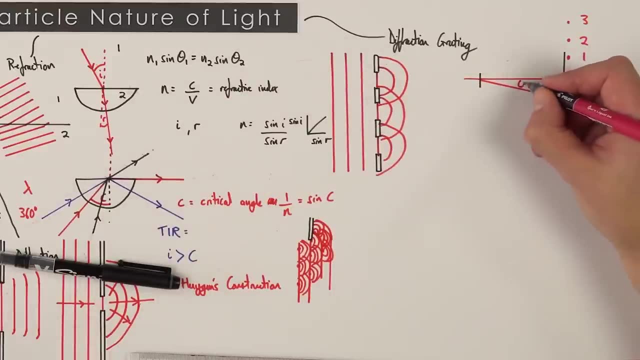 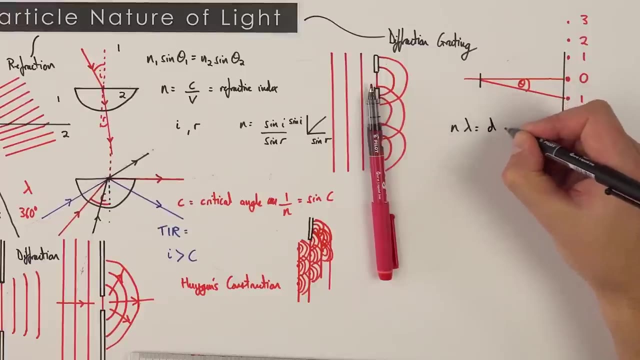 If we were to think about this, there's, as we follow this line back over here, the angle between the zeroth and the first order is equal to theta, and what we can say is that n lambda is equal to d sine theta, where n refers to the order of light that we're observing. So in this case, here we'd. 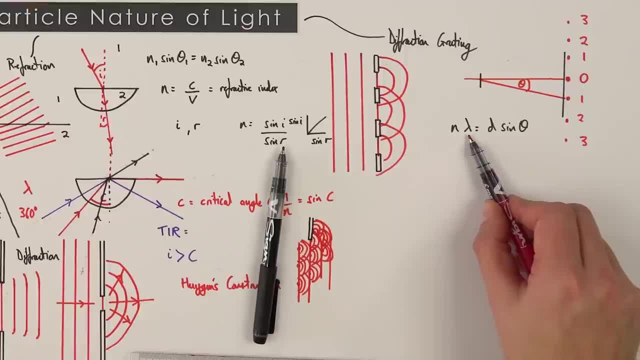 have theta and n would be equal to one, And you can see on the larger documents here that theta is due to the friendliness of the zone here n or n minus theta, and then the theta is due to the wavelength of that light. 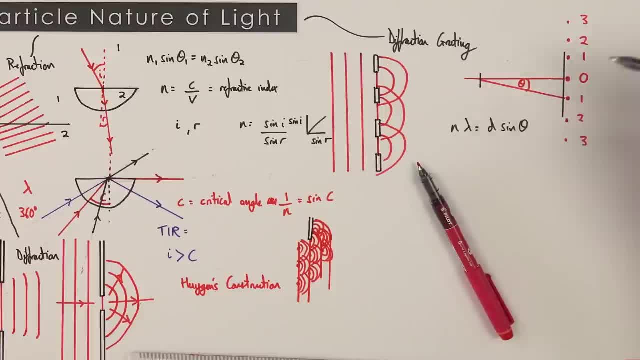 And d is the distance between the gratings on that diffraction grating. Now for something like this: how do you work out theta? Well, you could easily measure the distance from the diffraction grating to the screen. You can measure the distance between the bright. 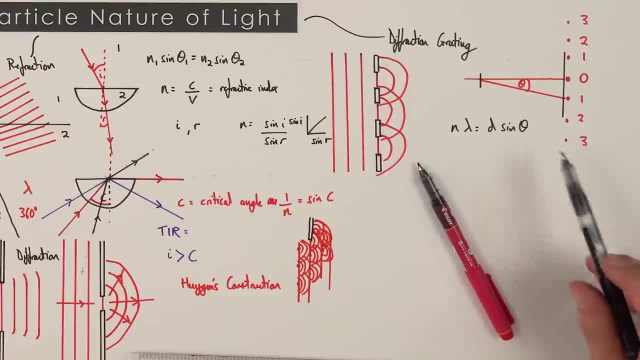 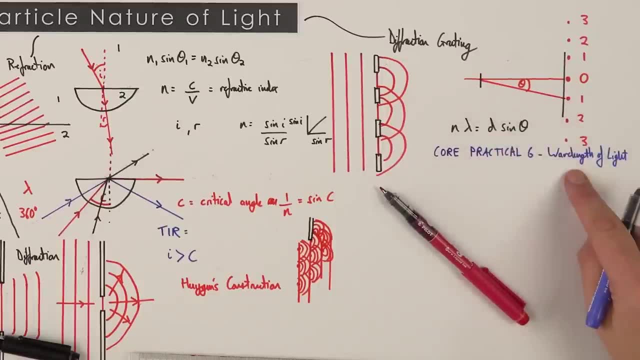 spots and then use a bit of trigonometry to work out the angle of theta And what you after seeing, is that theta's going to change. if we're thinking about n equals 2,, n equals 3, and so on, at core practical 6.. And this is looking at how you measure the wavelength of light. So if you know, 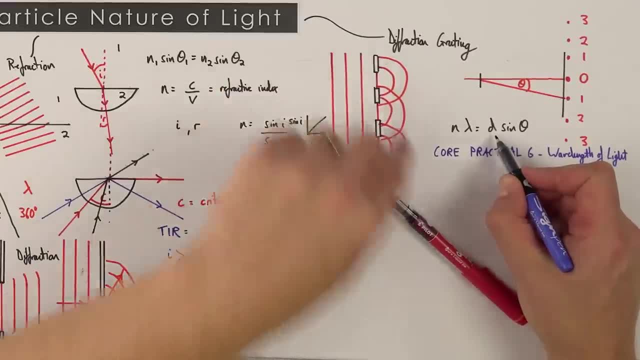 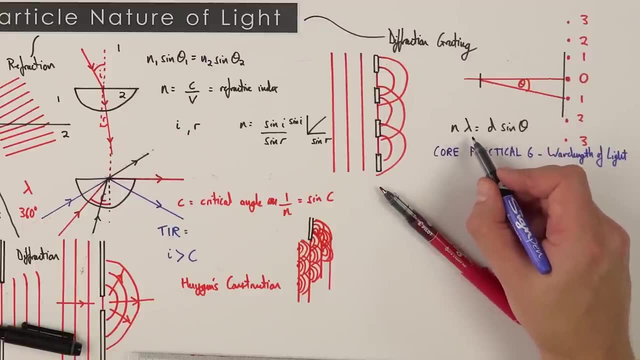 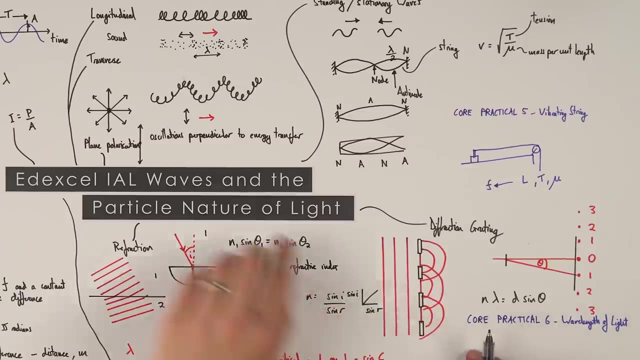 n. you can work out the distance between the diffraction gratings d. you can measure some other lengths to work out the value of theta. you can actually use this to work out the wavelength of light, which is going to be in the order of nanometres. Now the final thing, when it comes to 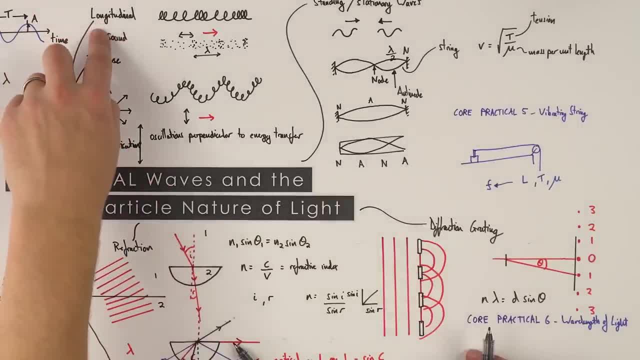 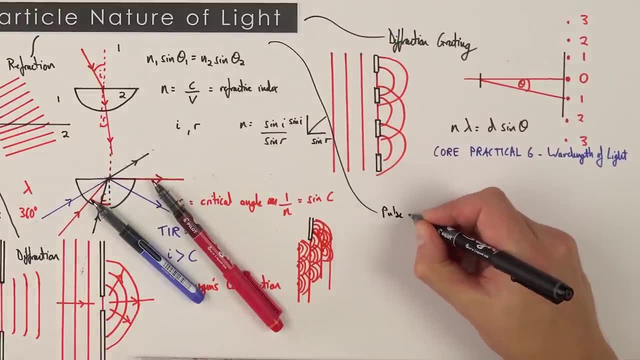 looking at the wave-like properties is if you had a longitudinal wave, perhaps sound or even ultrasound, what you can do. you can use this using a pulse echo technique to measure the distance to objects. Now, this is often used in scanning in medical uses because it's non-invasive. 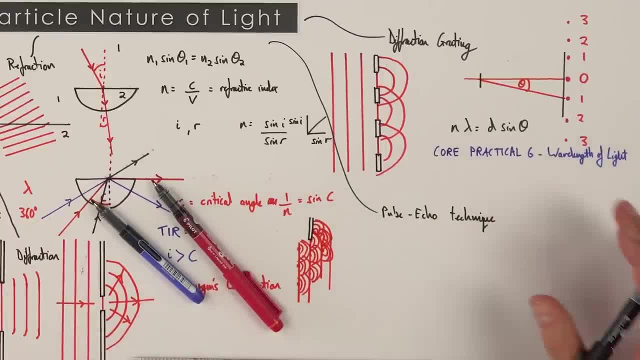 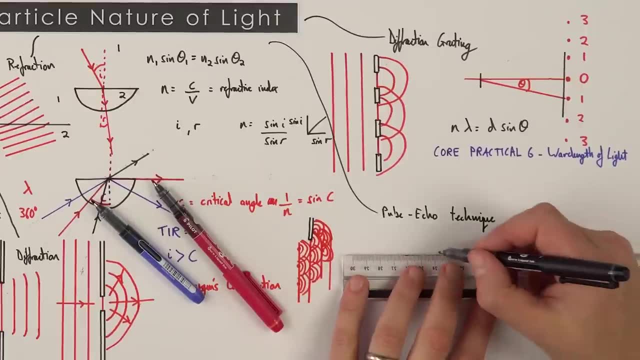 there's no ionising radiation, and you can use it to build up a picture of what's inside a person, including a developing foetus. Now let's think about a maybe more simple thing to do So. if you're looking at the wavelength of light, you can use this to 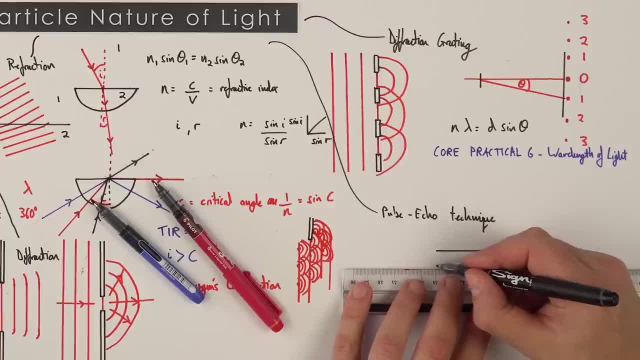 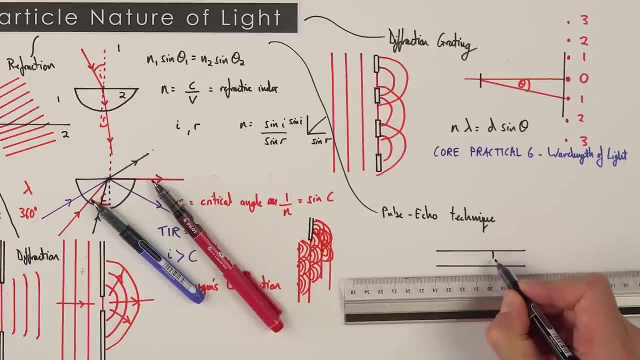 consider: maybe we had a length of pipe underground and it's very hard to actually go down and dig it up. But maybe there is a crack somewhere in a pipe, maybe it's a water pipe that's losing water. So this is the end of the pipe. at each end. Now, if you had some kind of 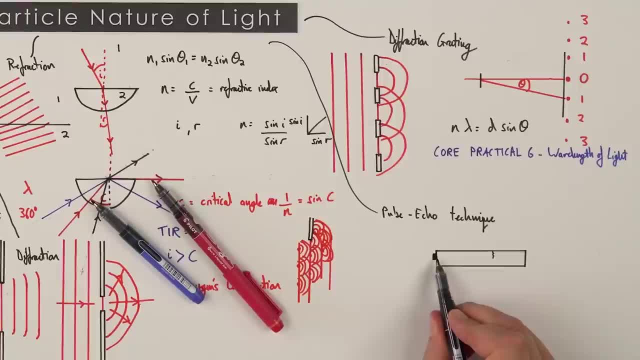 sensor here. what you could do is you could send a signal down the pipe and some of that signal is going to be reflected at a change in medium. Now here we've got a crack and we've got a crack, so it's going to be the pipe, a bit of air and then the pipe again. So what's going to? 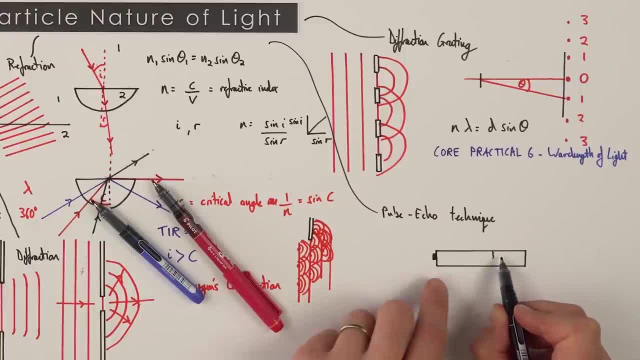 happen is, at this point here, some of that wave- perhaps we have an ultrasound wave- that's being emitted at this end. some of that wave is going to be reflected back here to the receiver and some of it's going to be transmitted through and maybe bounce back off the end of the pipe. Now what? this? 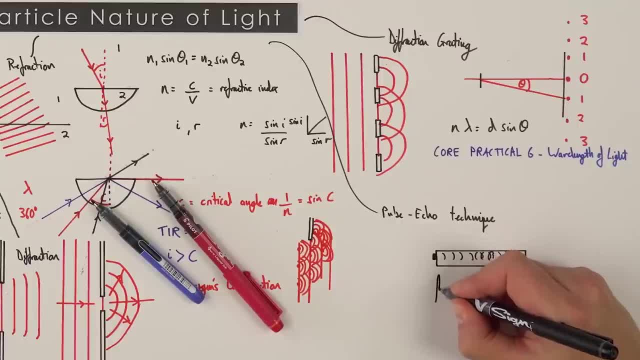 might look like is you maybe have an initial signal, which is your transmitted pulse, and then you receive a partial echo and then a short time later you receive a bit more of an echo. So here we have time along this axis here. if you were to imagine this on a graph, Now, in this very simple 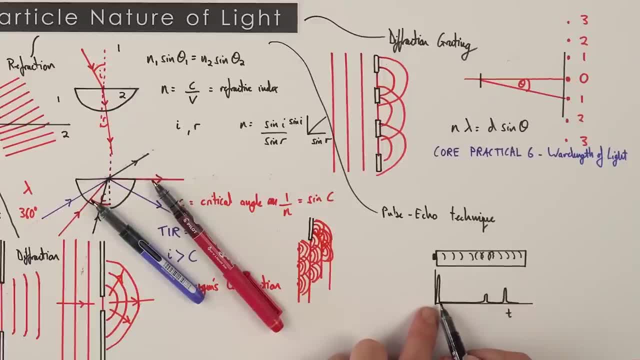 2D case. if you knew the time between the pulse being sent and received and you knew the speed of that wave and that material, then you could use these two bits of information to work out the distance to wherever that change in boundary might be. 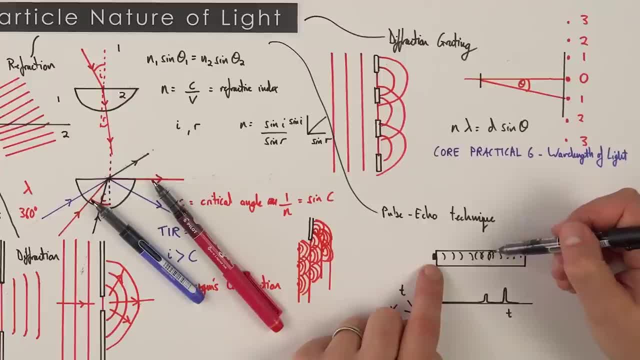 Now. this would then give you the distance to the pipe, so you know where to dig down and actually mend it. If you had lots of information like this, you could actually build up a 3D picture of what's going on. but really that's limited by perhaps the wavelength of the waves that you can actually use. 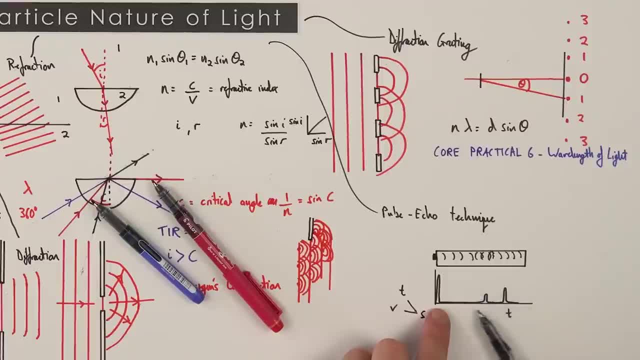 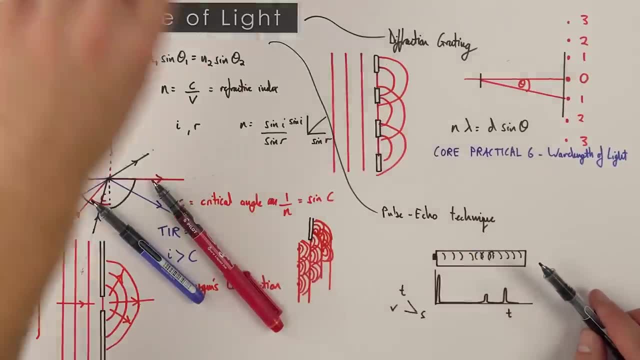 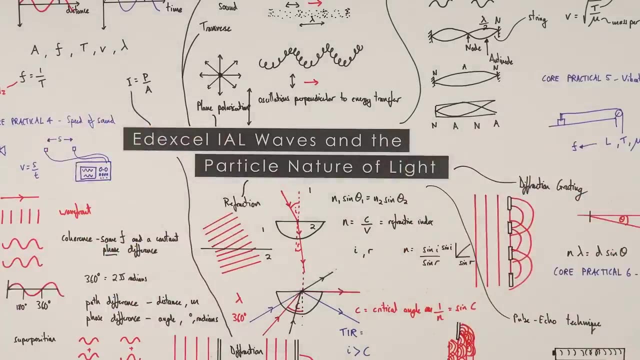 and also the duration of the pulse. So this thing here will give you a good indication of actually how to look inside an object. So that's the pulse echo technique, using, in this case, longitudinal mechanical waves. So a lot of information here about waves and the way that we can explain the behaviour of light. 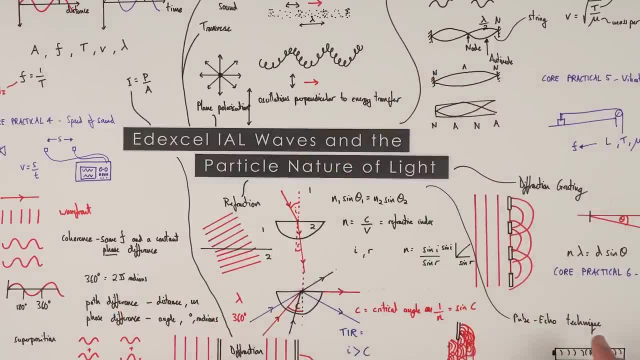 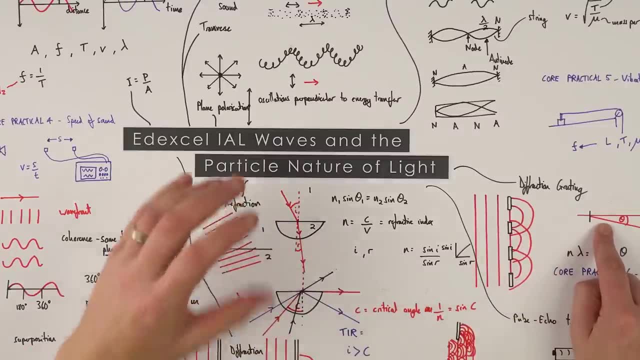 in terms of the wave model. However, we also found that some things which we often thought of as particles, like electrons, would actually diffract, And there are other things where the wave-like model of light couldn't explain the behaviour that we can actually see in real life. 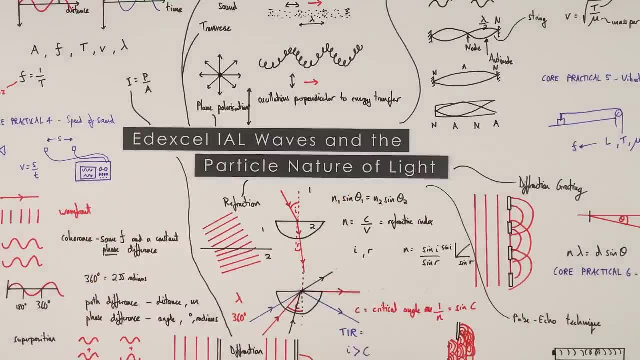 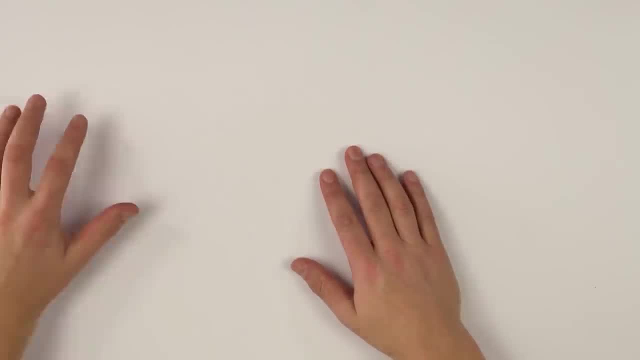 And that's why we're now going to look at the particle nature of light. I've kind of run out of paper here, so I'm just going to get another piece of paper, And the first thing we're going to be looking at is electron diffraction. Now, with electron diffraction, this is often carried out in an 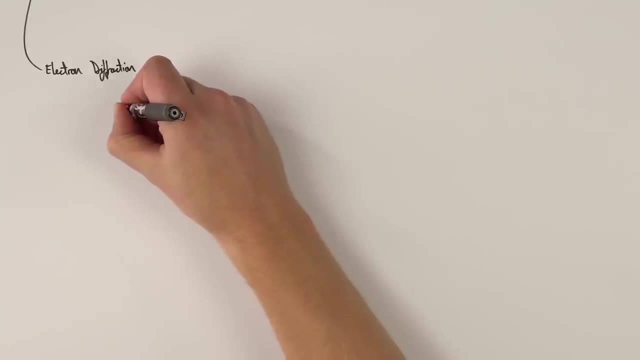 evacuated glass tube and that means that there's no air particles for the electrons to collide with. We have a cathode here at one end and at this cathode we can excite the electrons with a potential difference, and then we're going to have an anode over here which actually attracts. 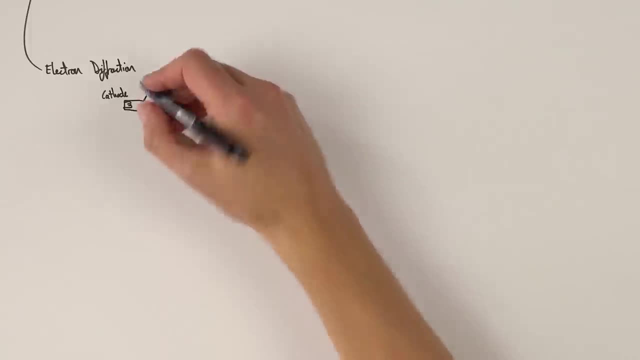 them. So that means we can accelerate electrons in this tube and what we're going to do is, at some point over here perhaps, we have a piece of graphite Now. graphite can be very thin and because it has the regular like arrangement of the carbon atoms inside, this graphite acts as 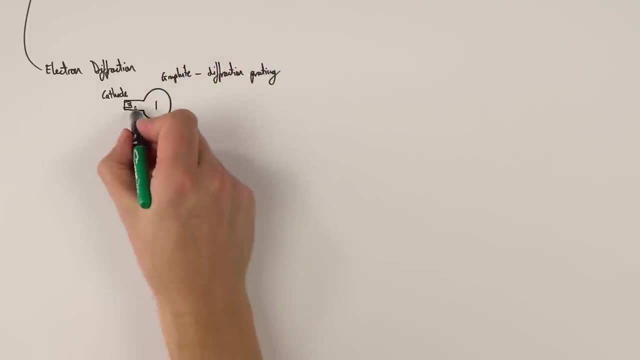 our diffraction grating and what we found was that when the electrons were accelerated and went through the graphite, we found that there was a diffraction pattern formed on the screen of the graphite. So we can see that there's a diffraction pattern formed on the screen of the 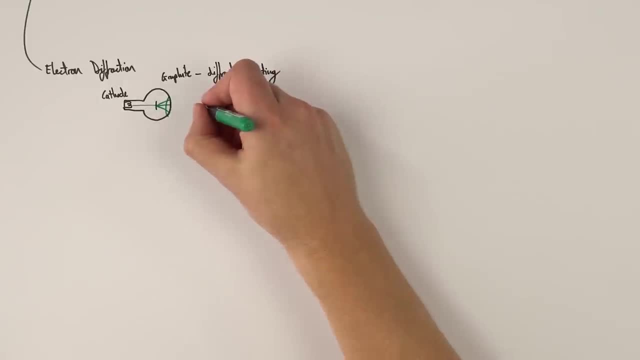 graphite and we can see that there's a diffraction pattern formed on the screen of the graphite over here. Now this is often covered in this phosphor coating and this glows where the electrons hit it. so we'd have like a central, like the zeroth order, and then we had concentric rings. 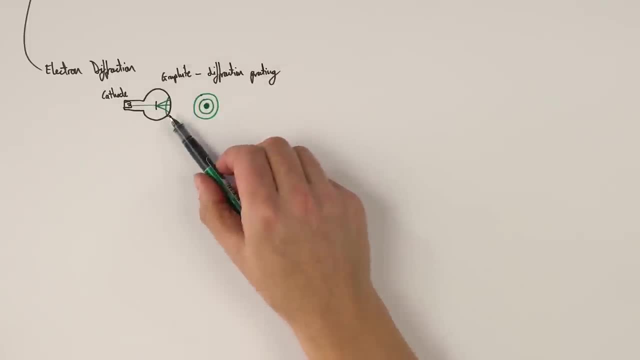 that show that actually the electrons as they pass through this graphite must be behaving like waves, because we have positions here where we have constructive interference and destructive interference, and the only way that we can explain this electron diffraction pattern is that electrons must be behaving with some wave-like properties. In actual fact, there's 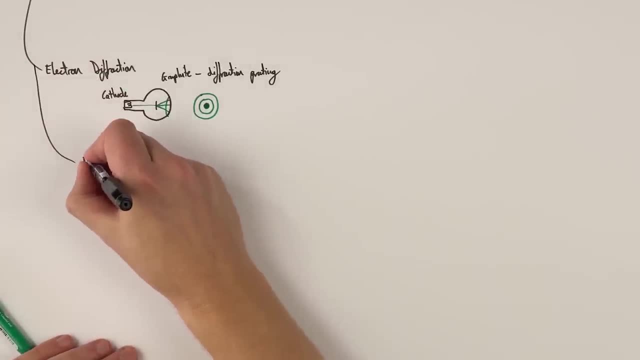 something called the de Broglie wavelength, and this means that the wavelength of that particle is going to be equal to h over p, where p is the momentum, and that really depends upon the mass of the particle and how quickly it's moving with its velocity. and here we've got. 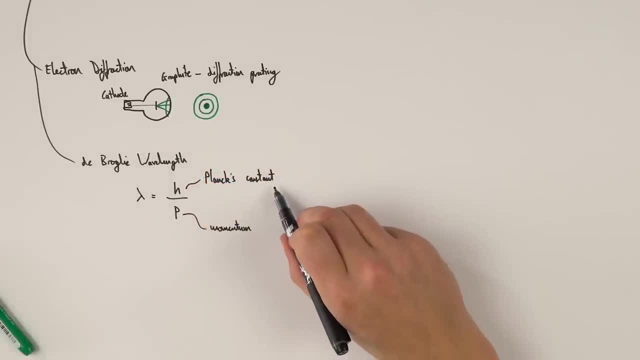 Planck's constant. and Planck's constant is equal to 6.626 times 10, to the minus 34.. So really, what this means is that even though we have the particle-like properties of something, where we know its mass and velocity, we can also then relate that to the wave-like properties of that particular. 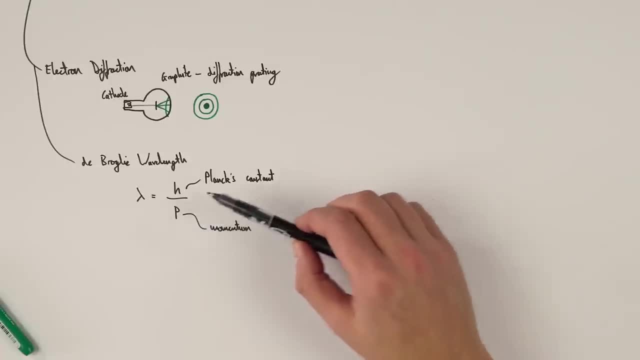 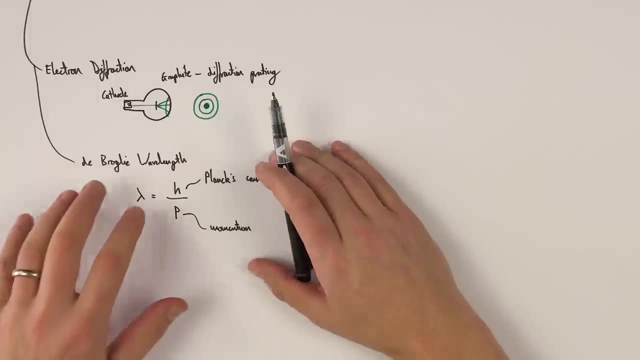 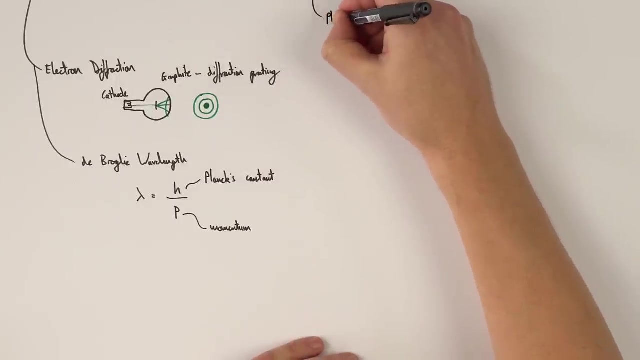 particle as it's travelling. So if we know the mass of an electron, we know how quickly it's travelling. that then tells us the electron's wavelength. So this is really looking at the wave-like properties of particles. but if we think about the particle-like properties of waves- a really good example of this- 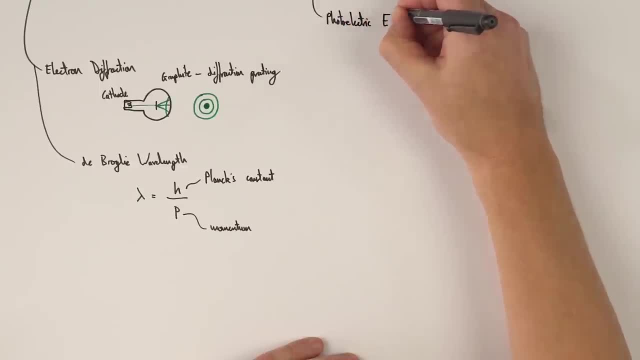 is something called the photoelectric effect, and here if you have the surface of a metal, if you shine light on it, then electrons will be emitted from that surface. Now, if you have a certain frequency of light, then that will allow these electrons to escape the surface. but below. 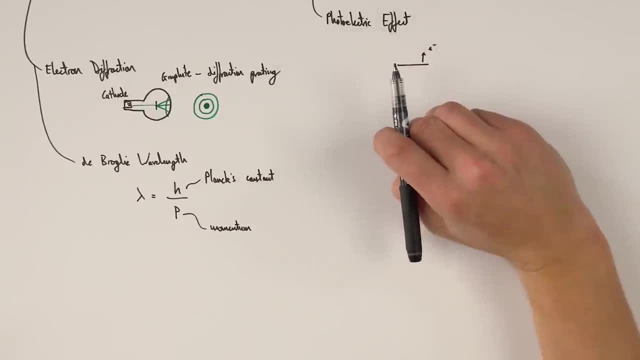 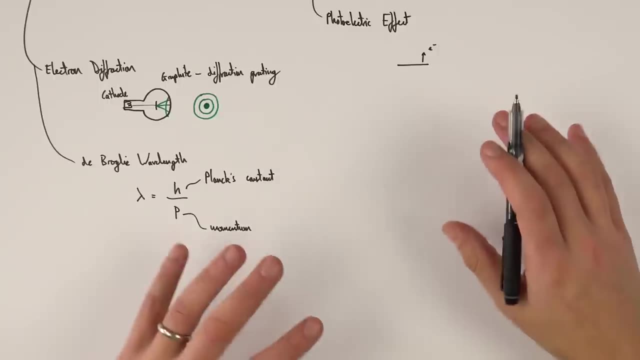 that frequency of light. there's a certain frequency of light that will allow these electrons to escape. nothing will be emitted. Now, this is one bit of evidence, which I'm going to come on to, about why light must have particle-like properties. The first thing I'm going to do, though, is just put 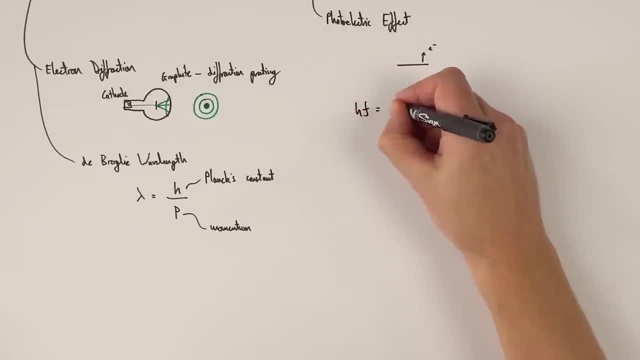 down this equation that says hf is equal to phi. so that's the greek letter, phi plus a half mv, max squared. Okay. so there's a lot to unpack, unpack in this. The first part here is due to the energy of these little packets of light that are incident on the surface, So I'm just going to draw a wave. 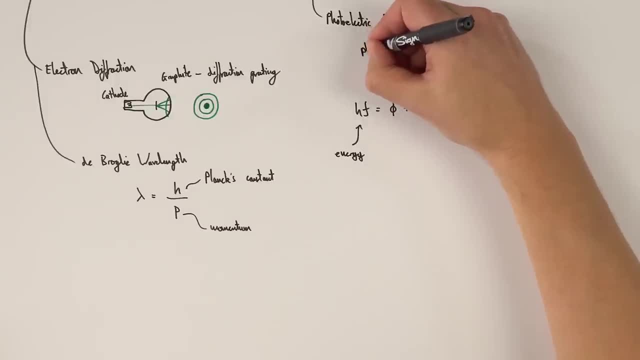 with an arrow to show that this is what we call a photon. Now, a photon is a little bundle of energy, so this hf here is equal to the energy of a photon, and we can say that e is equal to hf. Now h is Planck's constant that we saw over here, The energy of the photon really. depends upon the frequency. The higher the frequency of that light, the more energy it's transmitting or transferring. Now we might know about this already. We might have things like infrared, which is fairly low energy radiation, but as we go up through the EM spectrum, we 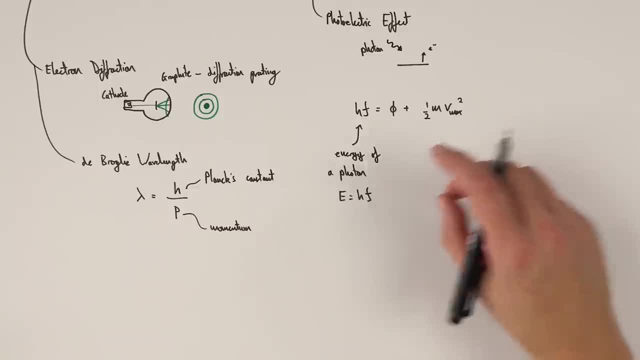 might have things like ultraviolet, which is more ionising. We then have x-rays and gamma rays and, as you have things which are a higher frequency, they carry more energy and that means it might be more ionising and potentially more dangerous to us. So this is the energy of the photon of light that is hitting that surface. Now that energy. 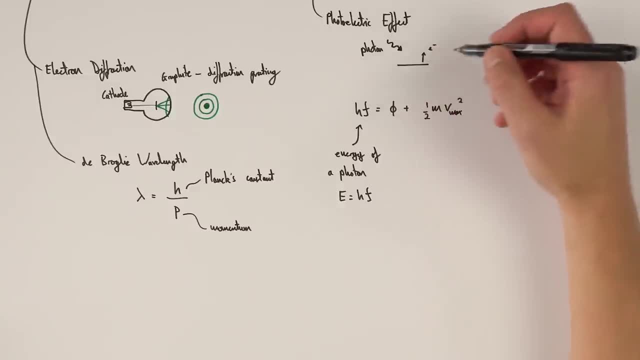 is going to be absorbed by electrons in the surface of this metal. and we have this thing here, phi, which we call the work function, And that's the energy required to take the electron out of that atom and away from the surface of that material. Now, any extra energy, 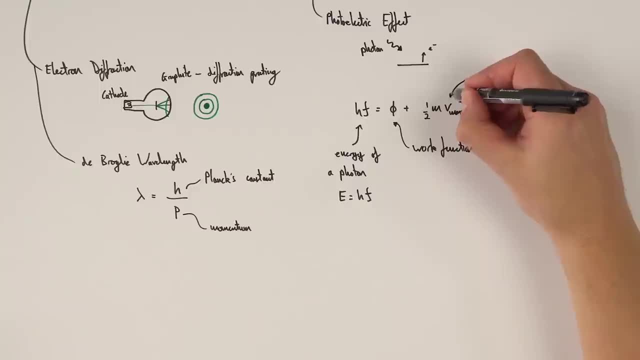 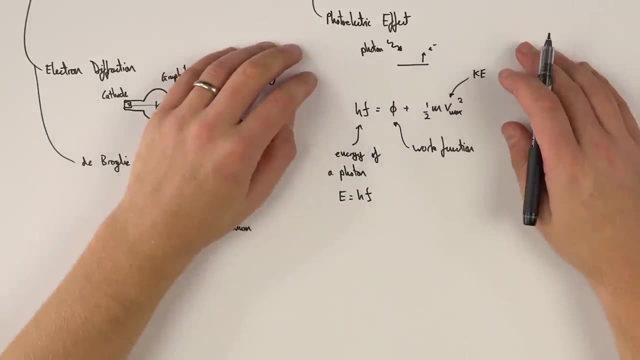 that's transferred to that electron is going to be in the photon and it's going to be in the light form of the kinetic energy of the emitted electrons. So the photoelectric effect is evidence for the particle-like nature of light. If you have a photon which is above the threshold, 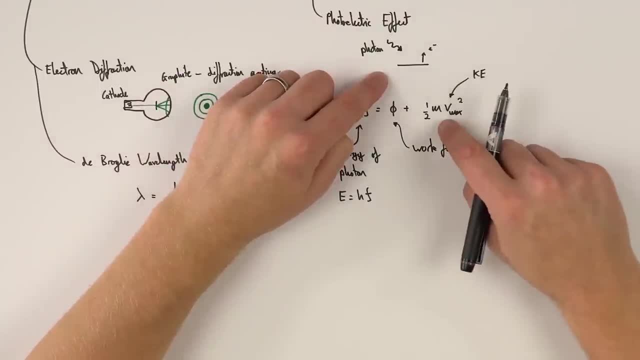 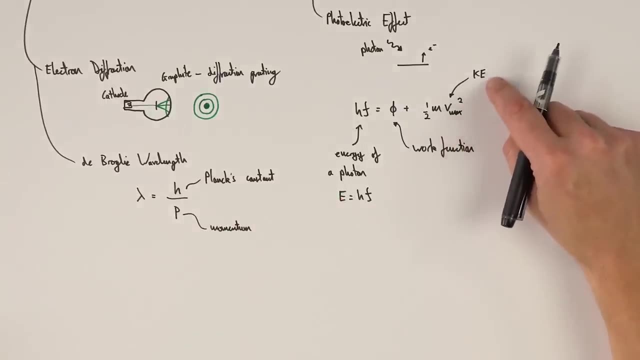 frequency that one photon absorbed by one electron will be emitted from the surface of that material and any extra energy transferred by that photon is going to end up in the kinetic energy stored by that particle as it moves off this photoelectron. Now this couldn't be explained. 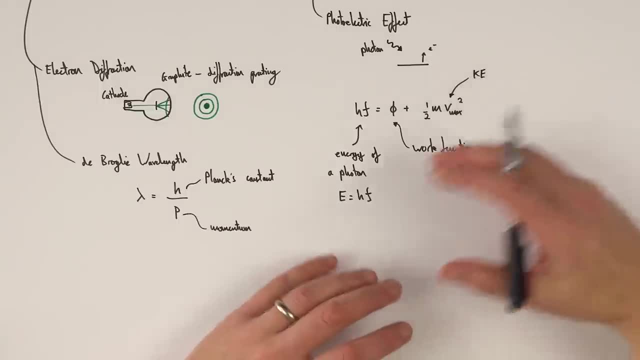 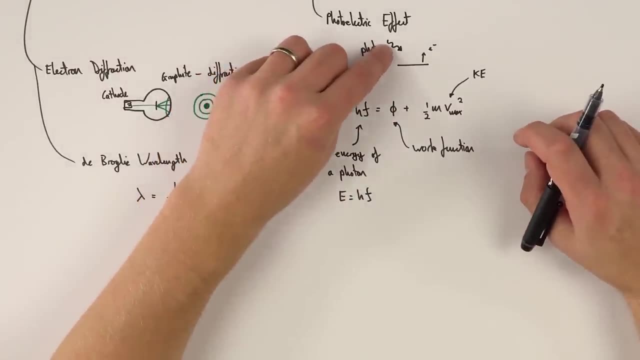 just by thinking about the wave-like properties of light. Otherwise, if you had something at a low frequency, perhaps red light, if you had really intense red light, then there should be enough energy being transferred to the surface to emit photoelectrons, But it's only above a certain 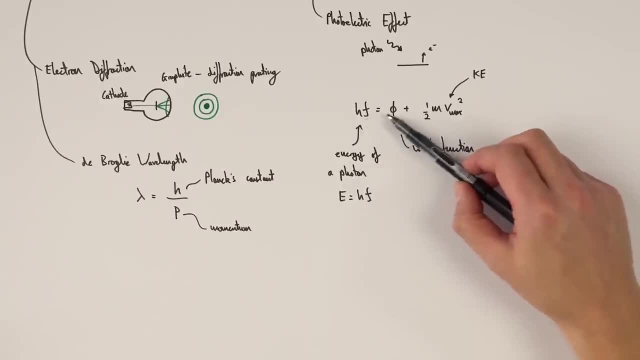 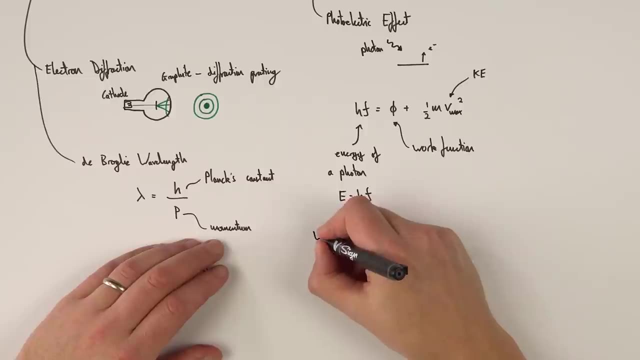 threshold frequency, that the photons have enough energy to be absorbed by the electrons and then the electrons to be emitted. And we can really bring these two things together when we consider wave-particle duality And basically, light has wave-like properties and it also has particle-like properties And 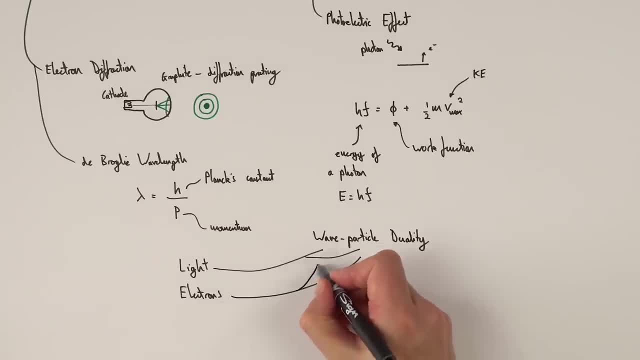 electrons, although we often consider them as particles, also have wave-like properties. In actual fact, the wave model and the particle model are just ways that we represent the behaviour of real things in physics. In reality, they're not perfectly a wave and they're not perfectly a. 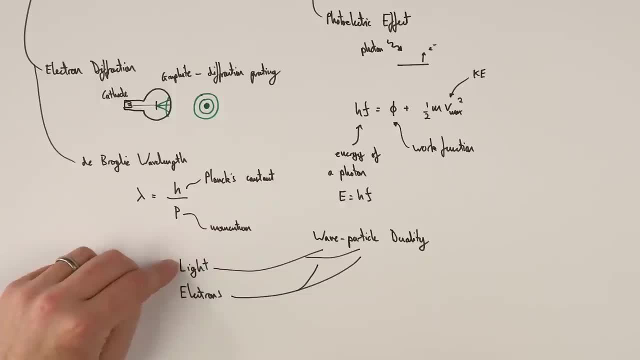 particle- They're a little bit of both- And light. it has wave-like properties, which explains things like diffusion and refraction, but it also has particle-like properties when we come to explain the photoelectric effect, Just like electrons have particle-like properties, often when we're 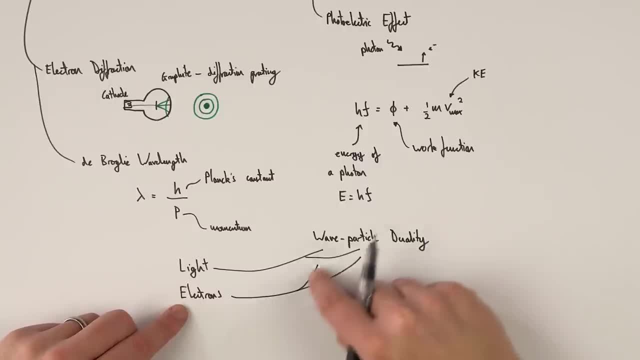 considering what's going on in chemistry. but they also have wave-like properties when they're travelling and that's how they can be diffracted. And just as an aside, because we're often considering maybe the energy of one electron, although usually we measure our energy in joules- 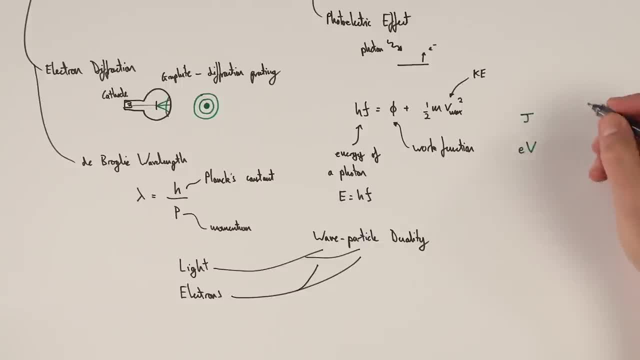 there's another unit called the electron volt. Now, an electron volt is the energy that's gained by one electron as it's accelerated through a potential difference of one volt. Now you might remember that E is equal to QV, The energy transferred is equal to the charge times, the 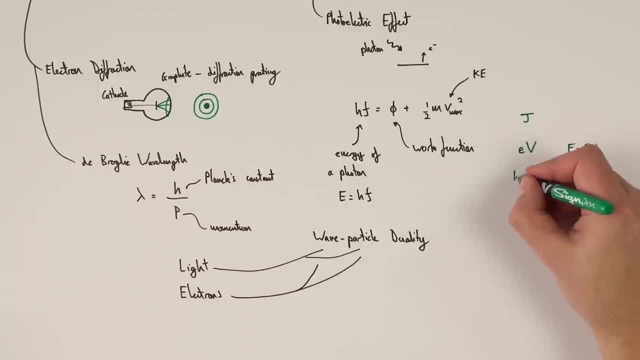 potential difference, And here that charge is going to be equal to 1.60 times 10 to the minus 19 coulombs. And if that was accelerated through a volt of exactly one, then we can say that one volt is equal to 1.60 times 10 to the minus 19 joules. So sometimes you'll be given data in 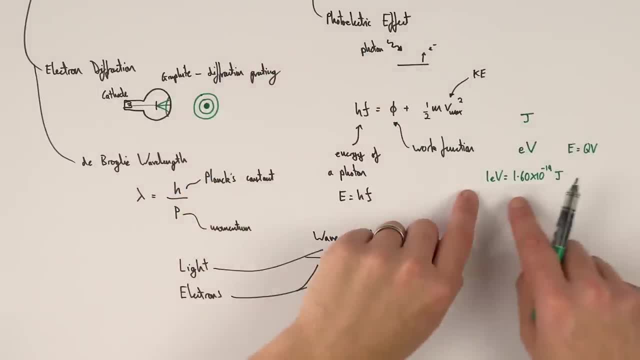 joules. sometimes you'll be given data in electron volts And it's good to be able to convert from one to the other. Now, the other thing in terms of like the way that photons and electrons can interact with each other is by looking at what actually happens within the different energy. 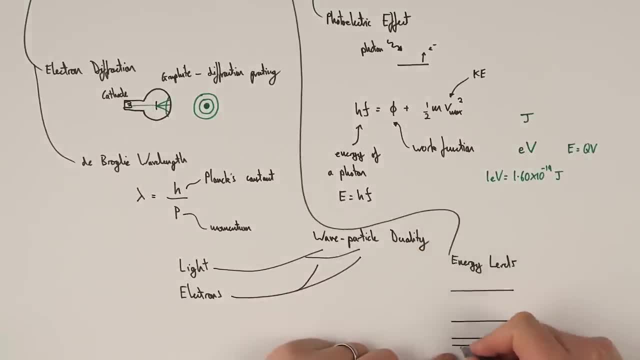 levels within an atom, Now often the electrons around the nucleus. they exist in what we call the ground state, But an electron could absorb a photon, So maybe we have a photon of light or some other sort of EM radiation And if it's exactly the right amount, the electron can jump up to another shell And 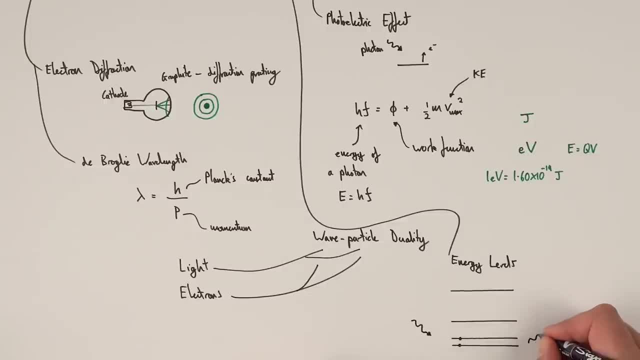 when the atom de-excites, this is going to jump back down and it's going to emit a photon of energy. So effectively, one photon absorbed by one electron. it jumps up an energy level and then, when it de-excites, it jumps back down. 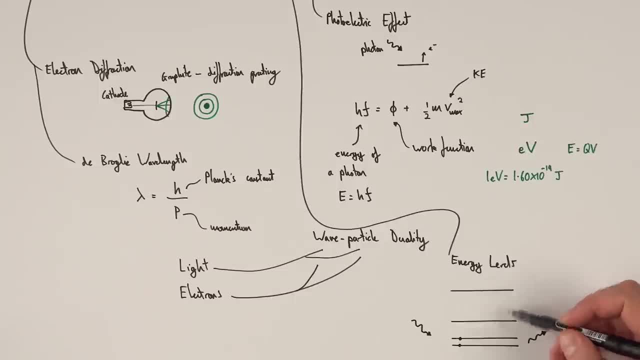 Now there are only distinct energy shells where an electron can exist. it could be a this one, or this one or this one. Now, sometimes we call these things like n equals one, equals two, three, up to the outermost shell, which is effectively infinity. Now the other thing we 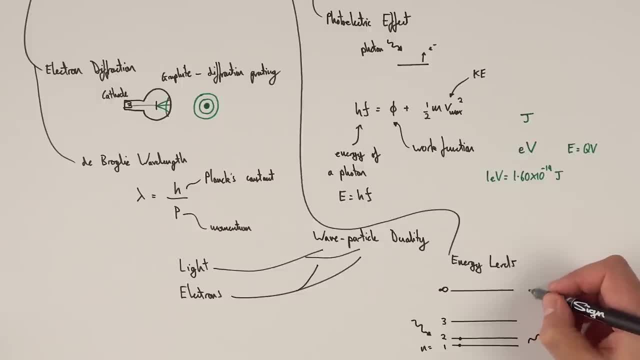 can do is we can give each of these a value of energy. So this one might be at 0.0, electron volts, one here might be minus 1.5 electron volts, minus 1.7 electron volts, and so on, And if you have any, 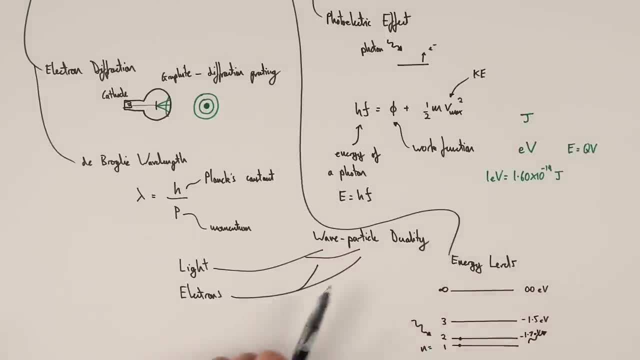 data like this. it'll be given to you in the question. But this means that we can actually calculate the energy of the photons which are either emitted or absorbed by the electrons in those energy levels. Now, perhaps an electron was excited to this shell. n equals 3. When it goes. 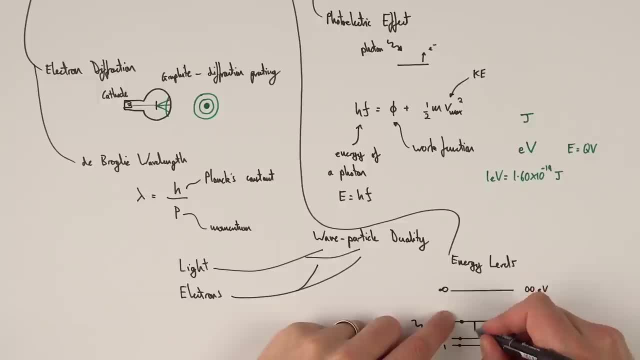 back down to the ground state. there's a couple of possibilities. It could drop like this: straight from 3 to 1, or it could go from 3 to 2, or it could go from 2 to 1.. And this means that there. 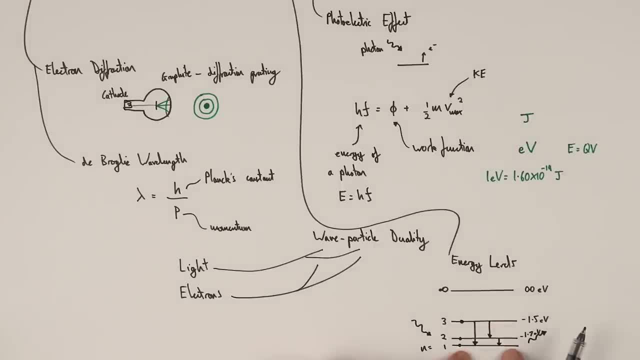 are three possible photons that could be emitted. that can actually be emitted And if you have any data like this, it'll be given to you in the question. only have a certain discrete amount of energy. If we wanted to look at this one here when it goes. 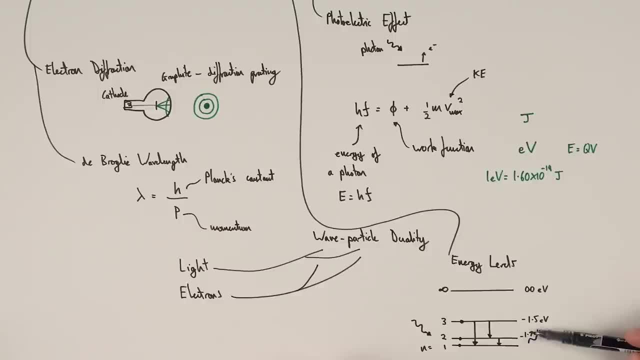 from 3 to 2,, it goes from minus 1.5 to minus 1.7. And that means the change is equal to 0.2 electron volts. Now, that's the energy of that photon. And because you can recall that E is, 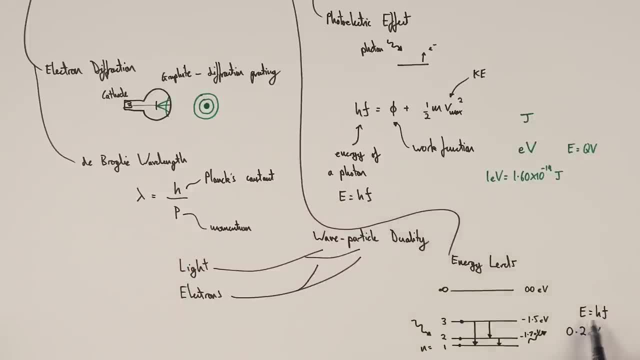 equal to HF up here. if we know the energy of that photon, we could work out the frequency of light that it would be emitting, And what we find is that the energy of that photon is different. So what we find is that different types of atoms or compounds have certain distinct